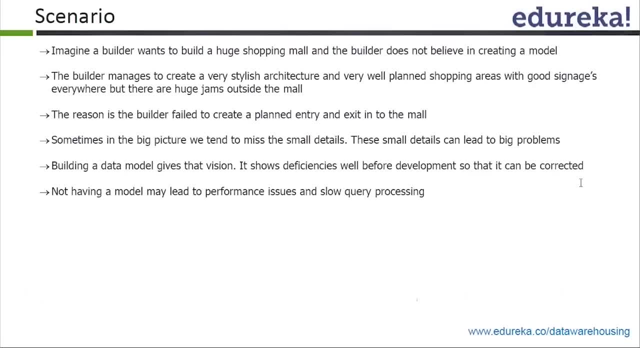 Our first slide, which gives us the scenario base for our discussion. So we just see this case study before we move on and see how to build a data warehouse for this particular case. So there is a builder who wants to build a huge shopping mall, right? So this scenario will actually help us to understand why exactly a model or a data model is important before we actually build a data warehouse or physical data warehouse. 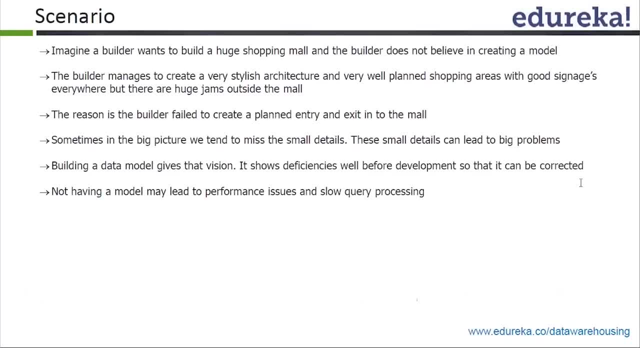 So in this case, there is a builder who wants to build a huge mall, but he wants to build a huge shopping mall. So he wants to build a huge shopping mall, So he wants to build a huge shopping mall. He doesn't. he just has a very stylish architecture and then he builds his mall without building a model or a physical model. So he actually didn't build a model before he built his building. 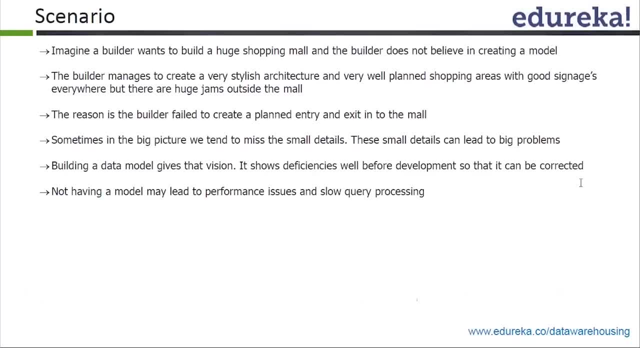 He had all the. he had nice architecture for his building, but he forgot to see that after he built his building he had all the. he had nice architecture for his building, but he forgot to see that after he built his building he had all the. he had nice architecture for his building, but he forgot to see that after he built his building. 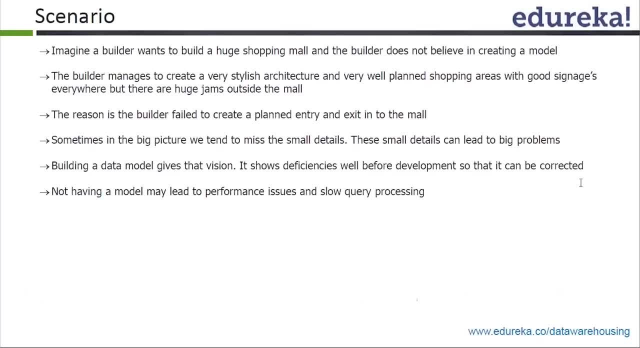 he sees that there is traffic jam outside his mall. So what exactly this situation says is that if he would have built a mall, maybe he would have seen the proper exit. he would have had a proper exit strategy for his mall. So what exactly this situation says is that if he would have built a mall, maybe he would have seen the proper exit strategy for his mall. 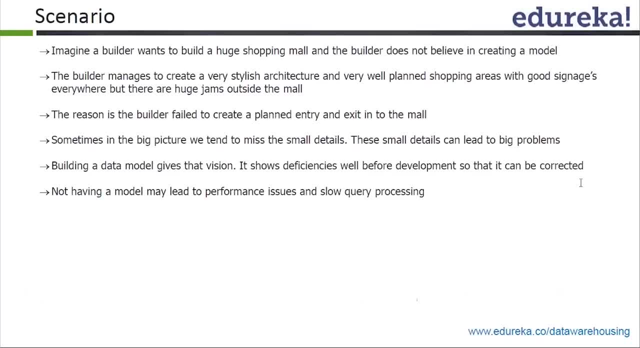 So what exactly this situation says is that if he would have built a mall, maybe he would have seen the proper exit strategy for his mall. So what exactly this situation says is that if he would have built a mall, maybe he would have seen the proper exit strategy for his mall. 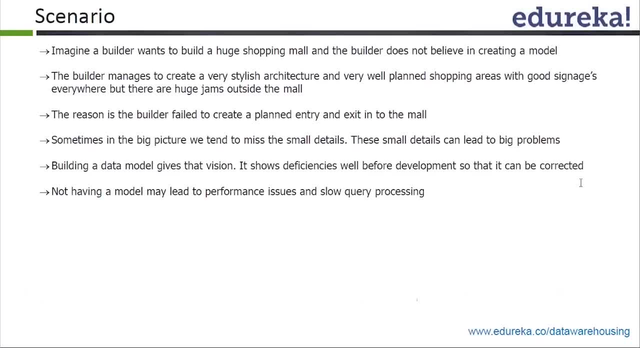 So what exactly this situation says is that if he would have built a mall, maybe he would have seen the proper exit strategy for his mall. So what exactly this situation says is that if he would have built a mall, maybe he would have seen the proper exit strategy for his mall. 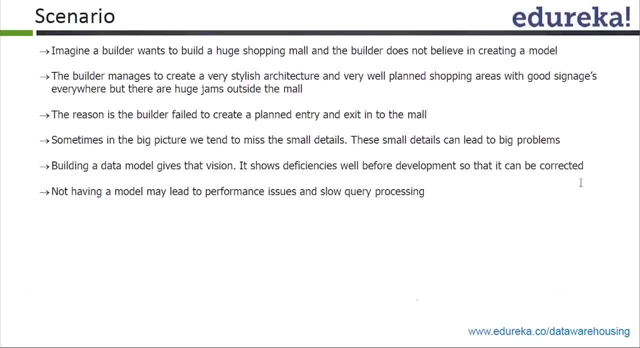 So what exactly this situation says is that if he would have built a mall, maybe he would have seen the proper exit strategy for his mall. So what exactly this situation says is that if he would have built a mall, maybe he would have seen the proper exit strategy for his mall. 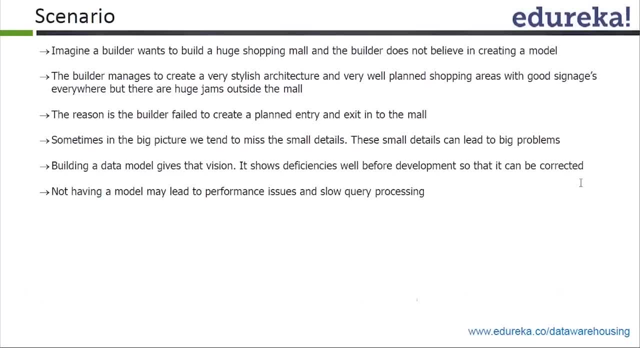 So what exactly this situation says is that if he would have built a mall, maybe he would have seen the proper exit strategy for his mall. So what exactly this situation says is that if he would have built a mall, maybe he would have seen the proper exit strategy for his mall. 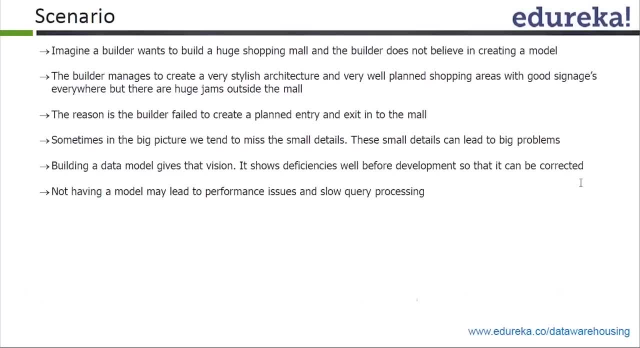 So what exactly this situation says is that if he would have built a mall, maybe he would have seen the proper exit strategy for his mall. So what exactly this situation says is that if he would have built a mall, maybe he would have seen the proper exit strategy for his mall. 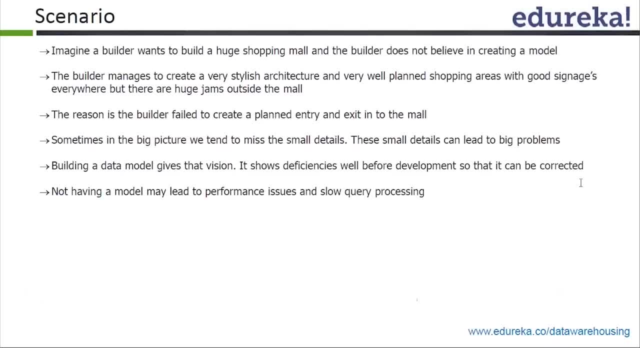 So what exactly this situation says is that if he would have built a mall, maybe he would have seen the proper exit strategy for his mall. So what exactly this situation says is that if he would have built a mall, maybe he would have seen the proper exit strategy for his mall. 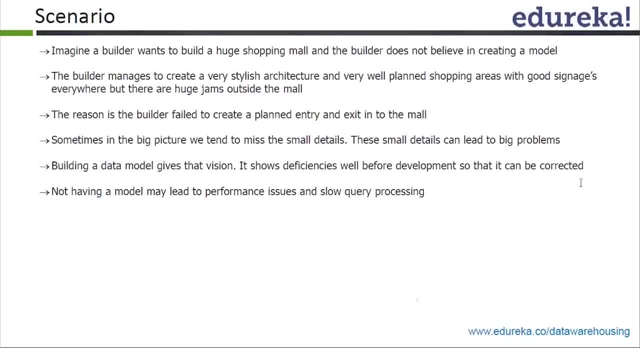 So what exactly this situation says is that if he would have built a mall, maybe he would have seen the proper exit strategy for his mall. So what exactly this situation says is that if he would have built a mall, maybe he would have seen the proper exit strategy for his mall. 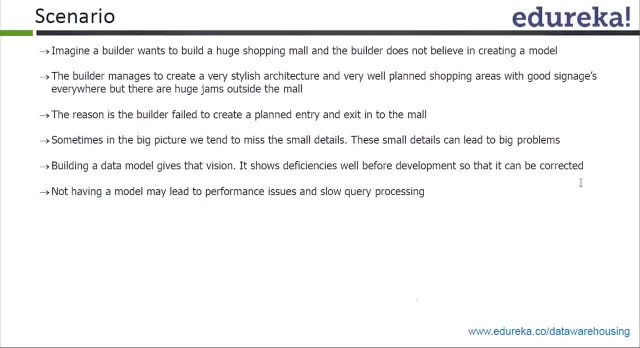 So what exactly this situation says is that if he would have built a mall, maybe he would have seen the proper exit strategy for his mall. So what exactly this situation says is that if he would have built a mall, maybe he would have seen the proper exit strategy for his mall. 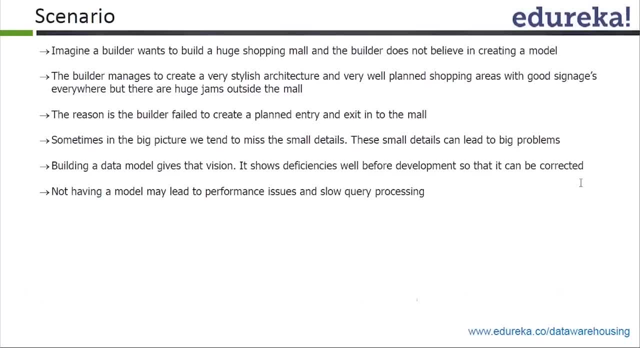 So what exactly this situation says is that if he would have built a mall, maybe he would have seen the proper exit strategy for his mall. So what exactly this situation says is that if he would have built a mall, maybe he would have seen the proper exit strategy for his mall. 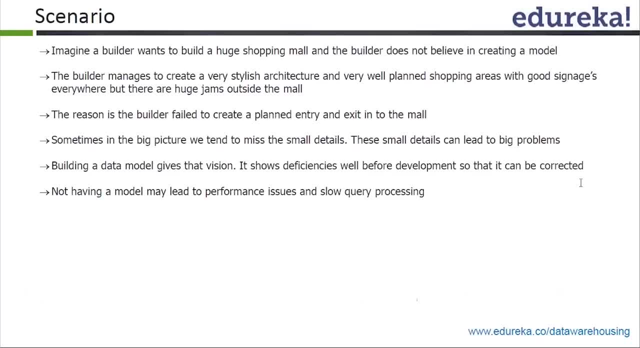 So what exactly this situation says is that if he would have built a mall, maybe he would have seen the proper exit strategy for his mall. So what exactly this situation says is that if he would have built a mall, maybe he would have seen the proper exit strategy for his mall. 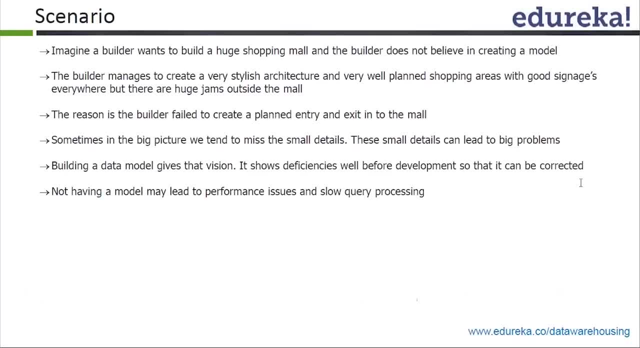 So what exactly this situation says is that if he would have built a mall, maybe he would have seen the proper exit strategy for his mall. So what exactly this situation says is that if he would have built a mall, maybe he would have seen the proper exit strategy for his mall. 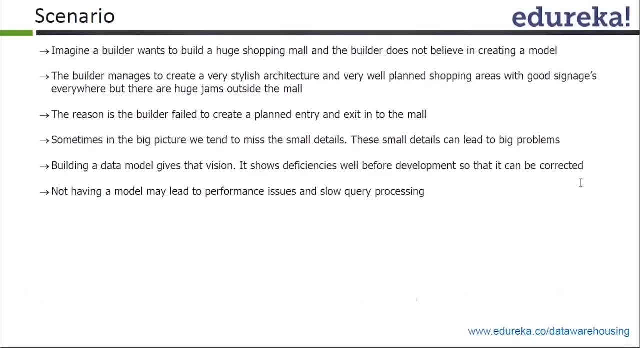 So what exactly this situation says is that if he would have built a mall, maybe he would have seen the proper exit strategy for his mall. So what exactly this situation says is that if he would have built a mall, maybe he would have seen the proper exit strategy for his mall. 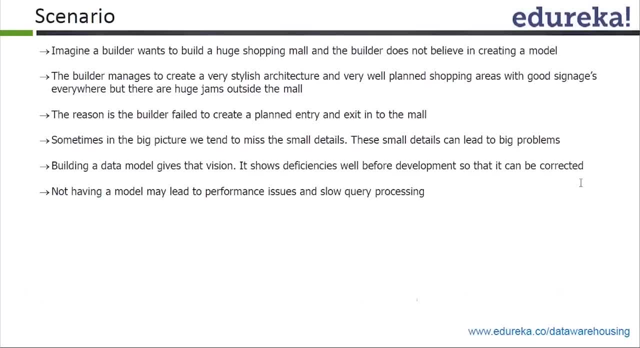 So what exactly this situation says is that if he would have built a mall, maybe he would have seen the proper exit strategy for his mall. So what exactly this situation says is that if he would have built a mall, maybe he would have seen the proper exit strategy for his mall. 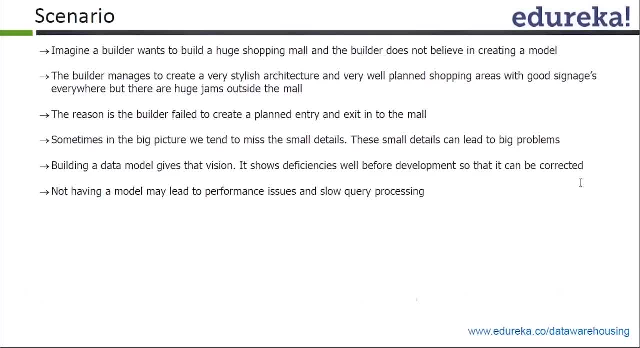 So what exactly this situation says is that if he would have built a mall, maybe he would have seen the proper exit strategy for his mall. So what exactly this situation says is that if he would have built a mall, maybe he would have seen the proper exit strategy for his mall. 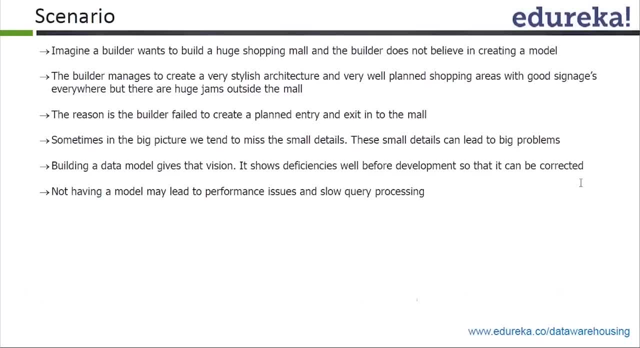 So what exactly this situation says is that if he would have built a mall, maybe he would have seen the proper exit strategy for his mall. So what exactly this situation says is that if he would have built a mall, maybe he would have seen the proper exit strategy for his mall. 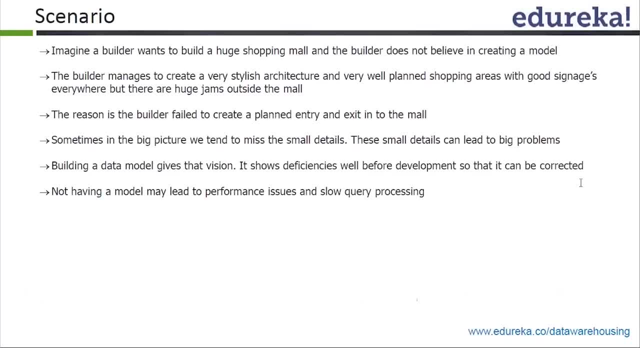 So what exactly this situation says is that if he would have built a mall, maybe he would have seen the proper exit strategy for his mall. So what exactly this situation says is that if he would have built a mall, maybe he would have seen the proper exit strategy for his mall. 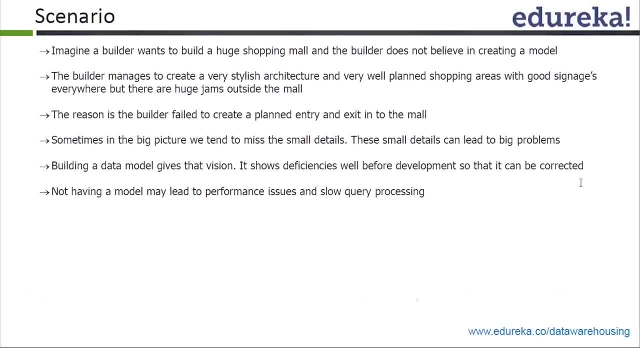 So what exactly this situation says is that if he would have built a mall, maybe he would have seen the proper exit strategy for his mall. So what exactly this situation says is that if he would have built a mall, maybe he would have seen the proper exit strategy for his mall. 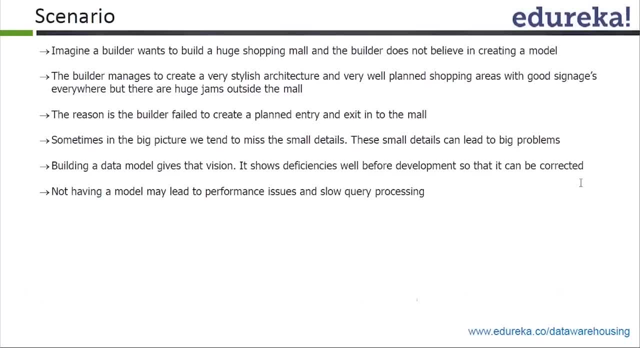 So what exactly this situation says is that if he would have built a mall, maybe he would have seen the proper exit strategy for his mall. So what exactly this situation says is that if he would have built a mall, maybe he would have seen the proper exit strategy for his mall. 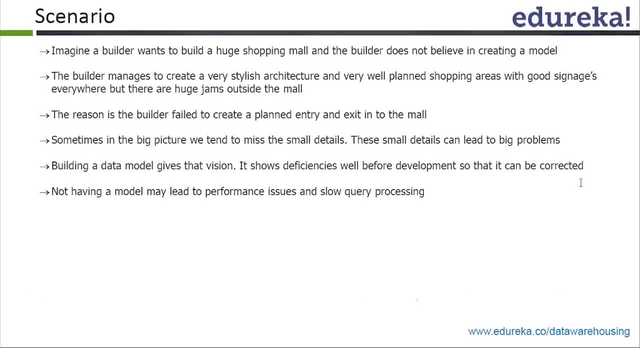 So what exactly this situation says is that if he would have built a mall, maybe he would have seen the proper exit strategy for his mall. So what exactly this situation says is that if he would have built a mall, maybe he would have seen the proper exit strategy for his mall. 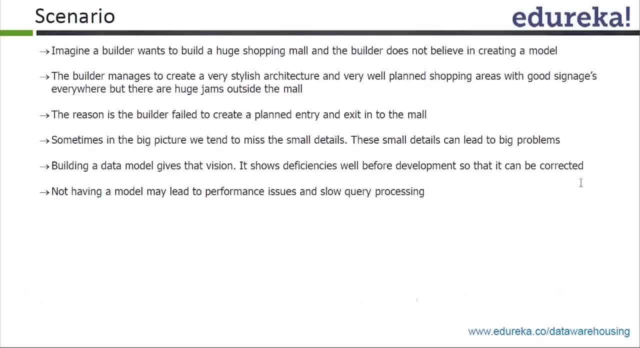 So what exactly this situation says is that if he would have built a mall, maybe he would have seen the proper exit strategy for his mall. So what exactly this situation says is that if he would have built a mall, maybe he would have seen the proper exit strategy for his mall. 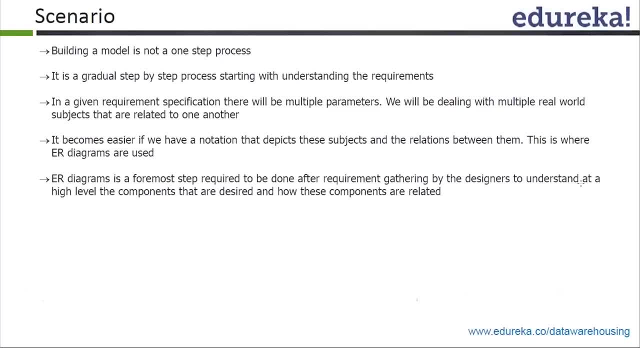 So what exactly this situation says is that if he would have built a mall, maybe he would have seen the proper exit strategy for his mall. So what exactly this situation says is that if he would have built a mall, maybe he would have seen the proper exit strategy for his mall. 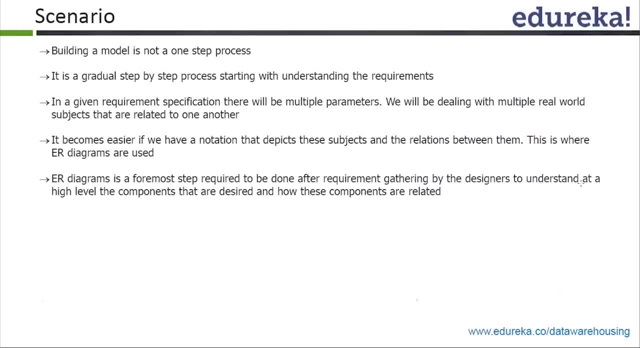 So what exactly this situation says is that if he would have built a mall, maybe he would have seen the proper exit strategy for his mall. So what exactly this situation says is that if he would have built a mall, maybe he would have seen the proper exit strategy for his mall. 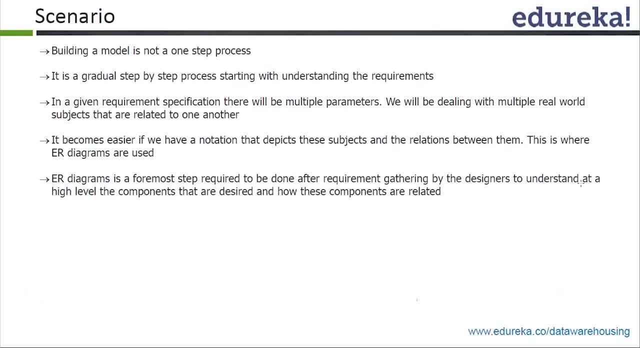 So what exactly this situation says is that if he would have built a mall, maybe he would have seen the proper exit strategy for his mall. So what exactly this situation says is that if he would have built a mall, maybe he would have seen the proper exit strategy for his mall. 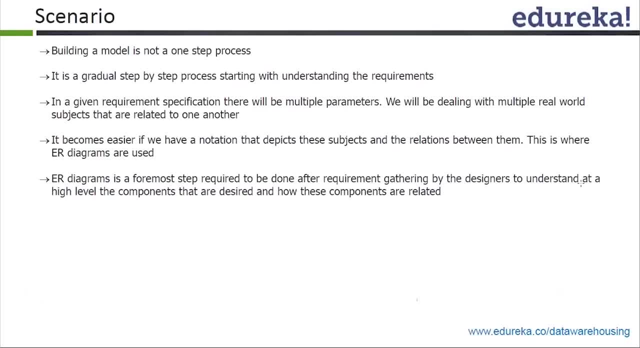 So what exactly this situation says is that if he would have built a mall, maybe he would have seen the proper exit strategy for his mall. So what exactly this situation says is that if he would have built a mall, maybe he would have seen the proper exit strategy for his mall. 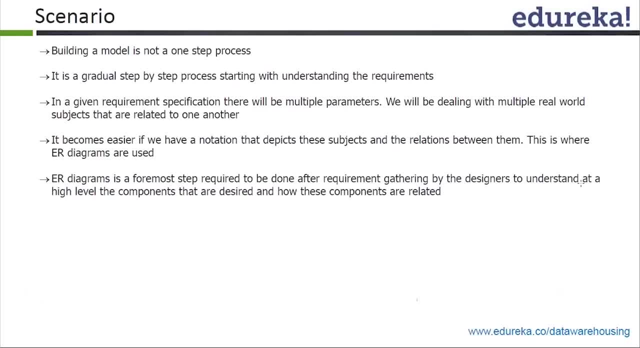 So what exactly this situation says is that if he would have built a mall, maybe he would have seen the proper exit strategy for his mall. So what exactly this situation says is that if he would have built a mall, maybe he would have seen the proper exit strategy for his mall. 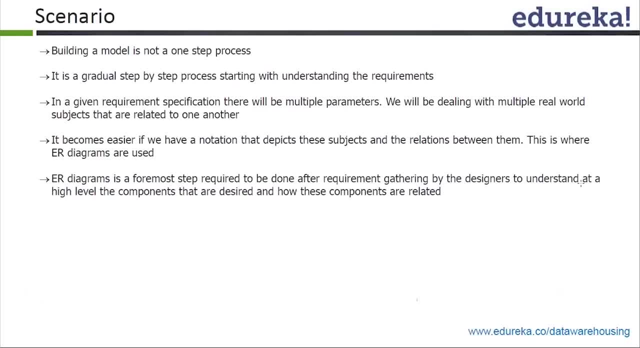 So what exactly this situation says is that if he would have built a mall, maybe he would have seen the proper exit strategy for his mall. So what exactly this situation says is that if he would have built a mall, maybe he would have seen the proper exit strategy for his mall. 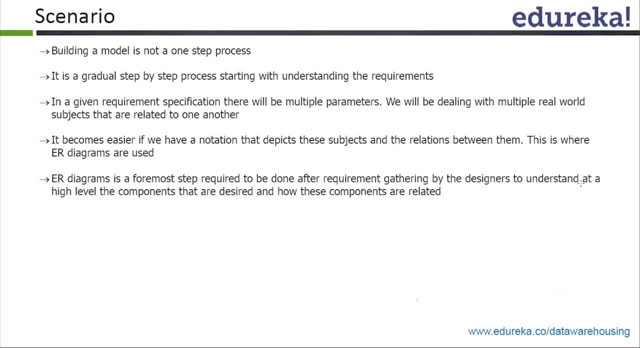 So what exactly this situation says is that if he would have built a mall, maybe he would have seen the proper exit strategy for his mall. So what exactly this situation says is that if he would have built a mall, maybe he would have seen the proper exit strategy for his mall. 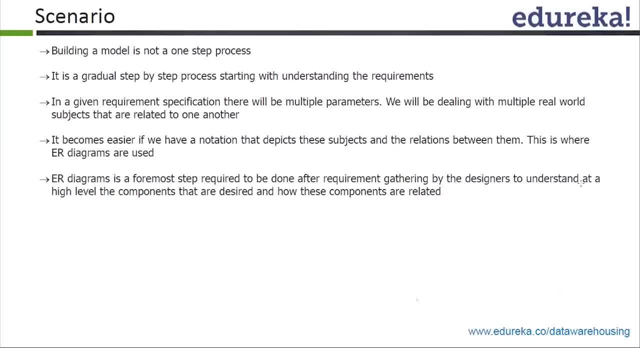 So what exactly this situation says is that if he would have built a mall, maybe he would have seen the proper exit strategy for his mall. So what exactly this situation says is that if he would have built a mall, maybe he would have seen the proper exit strategy for his mall. 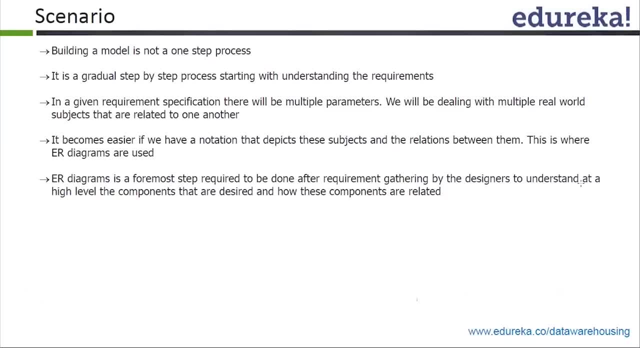 So what exactly this situation says is that if he would have built a mall, maybe he would have seen the proper exit strategy for his mall. So what exactly this situation says is that if he would have built a mall, maybe he would have seen the proper exit strategy for his mall. 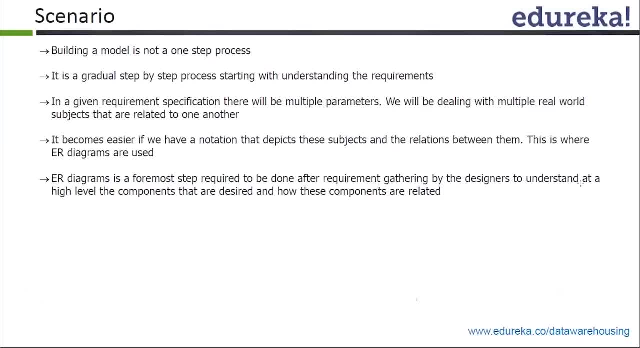 So what exactly this situation says is that if he would have built a mall, maybe he would have seen the proper exit strategy for his mall. So what exactly this situation says is that if he would have built a mall, maybe he would have seen the proper exit strategy for his mall. 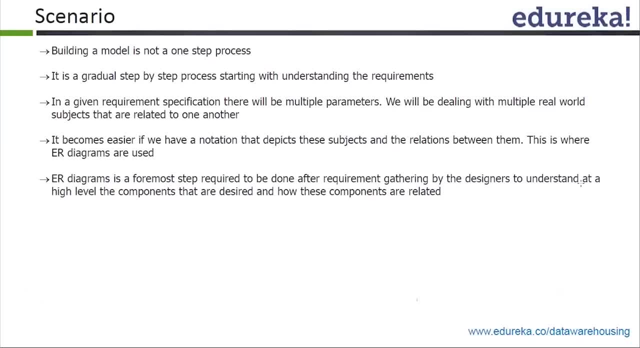 So what exactly this situation says is that if he would have built a mall, maybe he would have seen the proper exit strategy for his mall. So what exactly this situation says is that if he would have built a mall, maybe he would have seen the proper exit strategy for his mall. 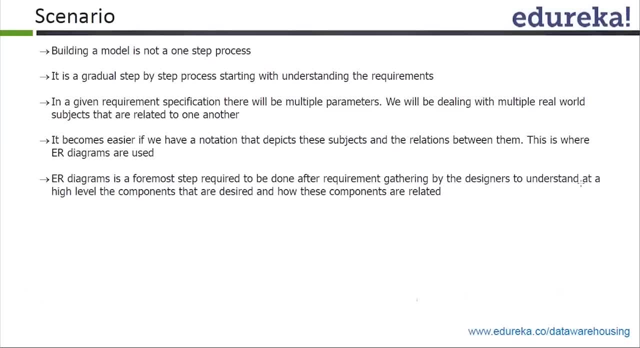 So what exactly this situation says is that if he would have built a mall, maybe he would have seen the proper exit strategy for his mall. So what exactly this situation says is that if he would have built a mall, maybe he would have seen the proper exit strategy for his mall. 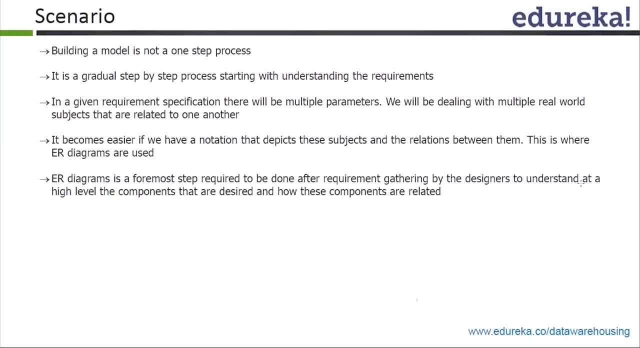 So what exactly this situation says is that if he would have built a mall, maybe he would have seen the proper exit strategy for his mall. So what exactly this situation says is that if he would have built a mall, maybe he would have seen the proper exit strategy for his mall. 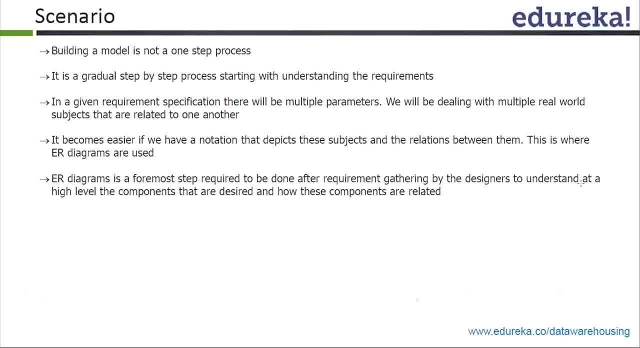 So what exactly this situation says is that if he would have built a mall, maybe he would have seen the proper exit strategy for his mall. So what exactly this situation says is that if he would have built a mall, maybe he would have seen the proper exit strategy for his mall. 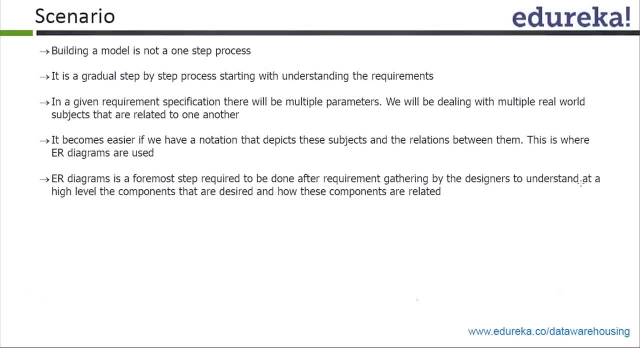 So what exactly this situation says is that if he would have built a mall, maybe he would have seen the proper exit strategy for his mall. So what exactly this situation says is that if he would have built a mall, maybe he would have seen the proper exit strategy for his mall. 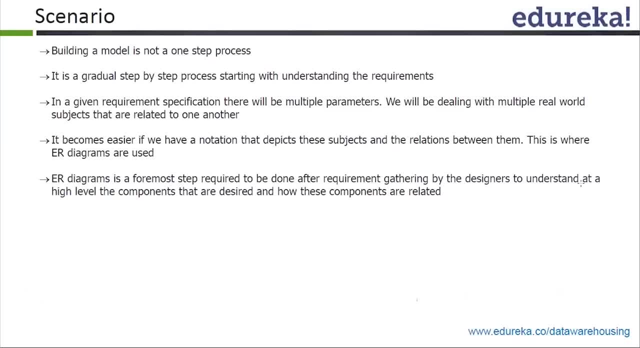 So what exactly this situation says is that if he would have built a mall, maybe he would have seen the proper exit strategy for his mall. So what exactly this situation says is that if he would have built a mall, maybe he would have seen the proper exit strategy for his mall. 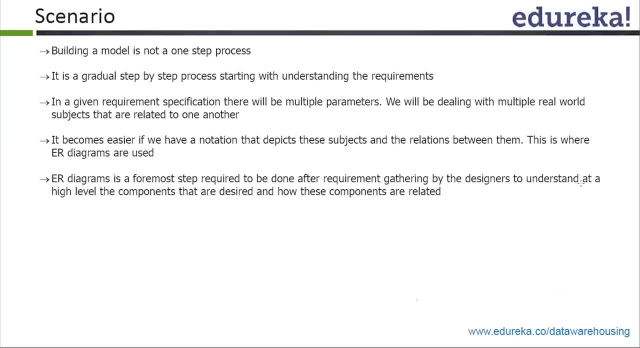 So what exactly this situation says is that if he would have built a mall, maybe he would have seen the proper exit strategy for his mall. So what exactly this situation says is that if he would have built a mall, maybe he would have seen the proper exit strategy for his mall. 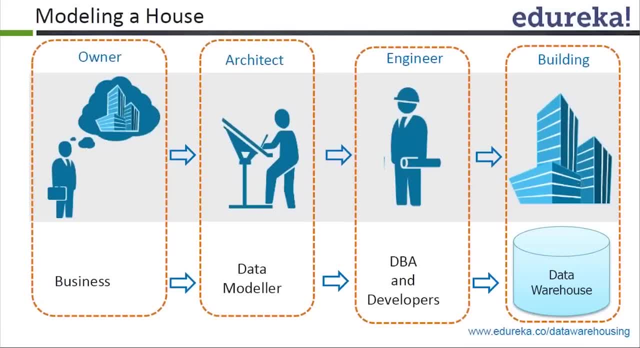 So what exactly this situation says is that if he would have built a mall, maybe he would have seen the proper exit strategy for his mall. So what exactly this situation says is that if he would have built a mall, maybe he would have seen the proper exit strategy for his mall. 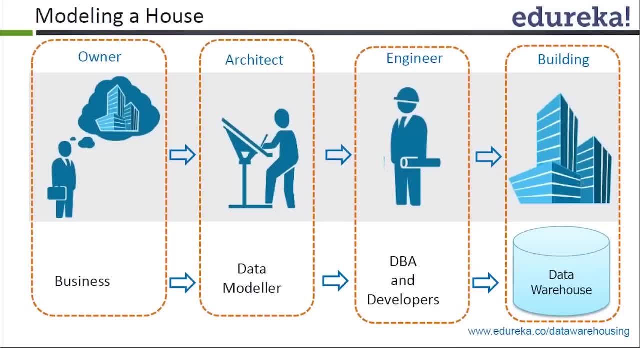 So what exactly this situation says is that if he would have built a mall, maybe he would have seen the proper exit strategy for his mall. So what exactly this situation says is that if he would have built a mall, maybe he would have seen the proper exit strategy for his mall. 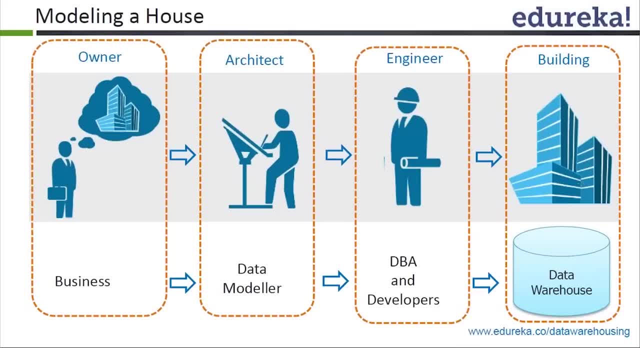 So what exactly this situation says is that if he would have built a mall, maybe he would have seen the proper exit strategy for his mall. So what exactly this situation says is that if he would have built a mall, maybe he would have seen the proper exit strategy for his mall. 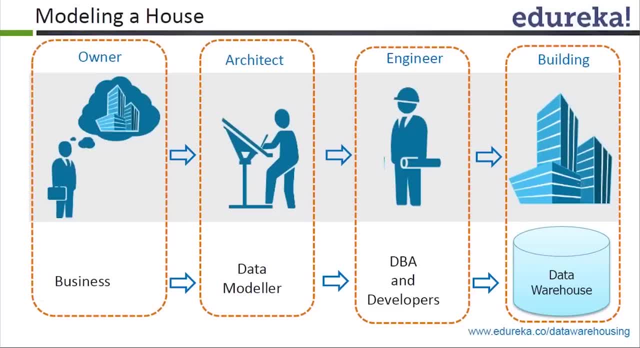 So what exactly this situation says is that if he would have built a mall, maybe he would have seen the proper exit strategy for his mall. So what exactly this situation says is that if he would have built a mall, maybe he would have seen the proper exit strategy for his mall. 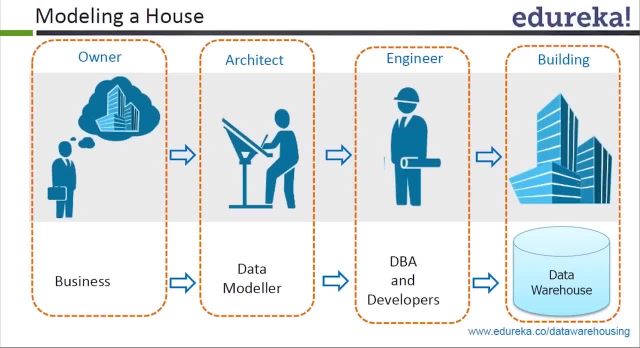 So what exactly this situation says is that if he would have built a mall, maybe he would have seen the proper exit strategy for his mall. So what exactly this situation says is that if he would have built a mall, maybe he would have seen the proper exit strategy for his mall. 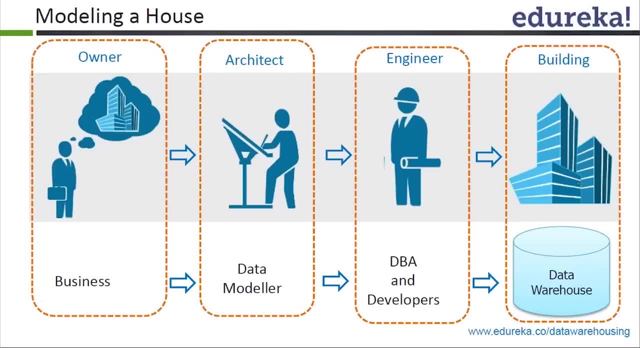 So what exactly this situation says is that if he would have built a mall, maybe he would have seen the proper exit strategy for his mall. So what exactly this situation says is that if he would have built a mall, maybe he would have seen the proper exit strategy for his mall. 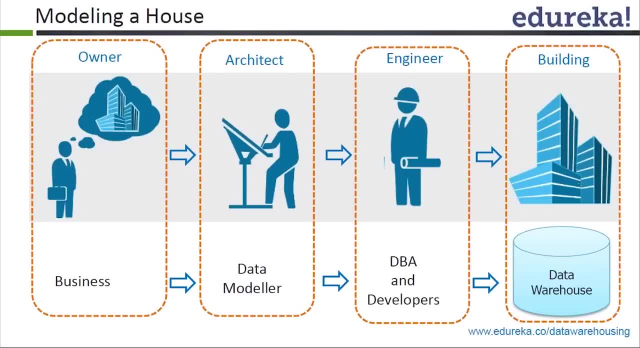 So what exactly this situation says is that if he would have built a mall, maybe he would have seen the proper exit strategy for his mall. So what exactly this situation says is that if he would have built a mall, maybe he would have seen the proper exit strategy for his mall. 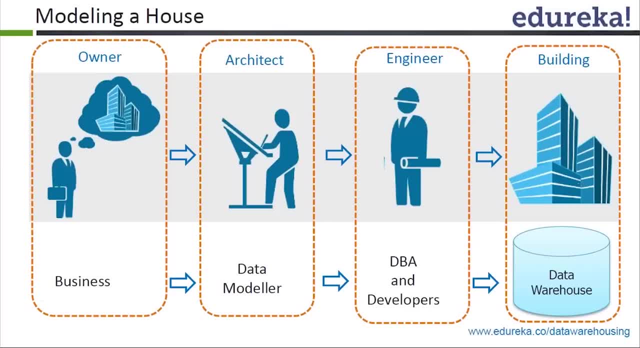 So what exactly this situation says is that if he would have built a mall, maybe he would have seen the proper exit strategy for his mall. So what exactly this situation says is that if he would have built a mall, maybe he would have seen the proper exit strategy for his mall. 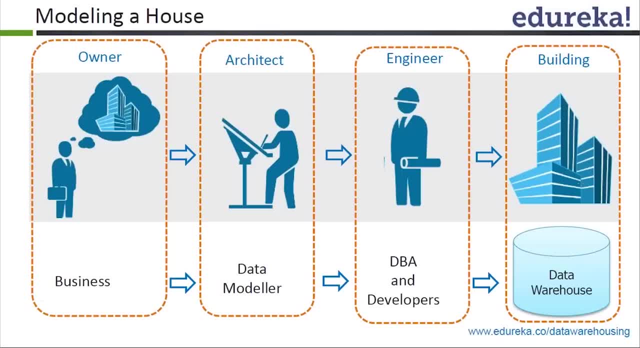 So what exactly this situation says is that if he would have built a mall, maybe he would have seen the proper exit strategy for his mall. So what exactly this situation says is that if he would have built a mall, maybe he would have seen the proper exit strategy for his mall. 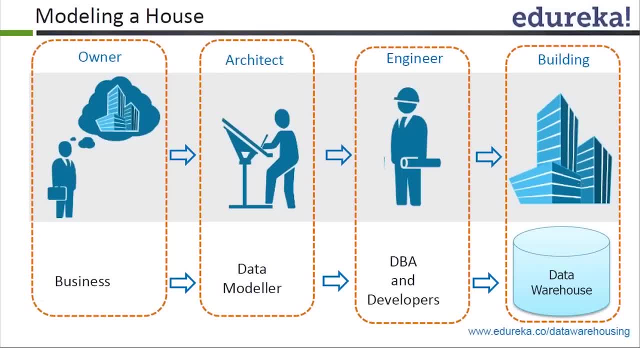 So what exactly this situation says is that if he would have built a mall, maybe he would have seen the proper exit strategy for his mall. So what exactly this situation says is that if he would have built a mall, maybe he would have seen the proper exit strategy for his mall. 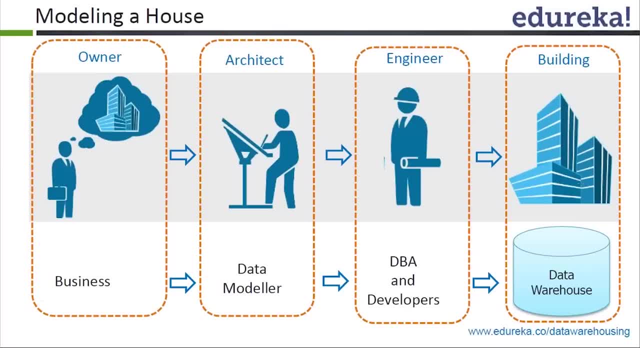 So what exactly this situation says is that if he would have built a mall, maybe he would have seen the proper exit strategy for his mall. So what exactly this situation says is that if he would have built a mall, maybe he would have seen the proper exit strategy for his mall. 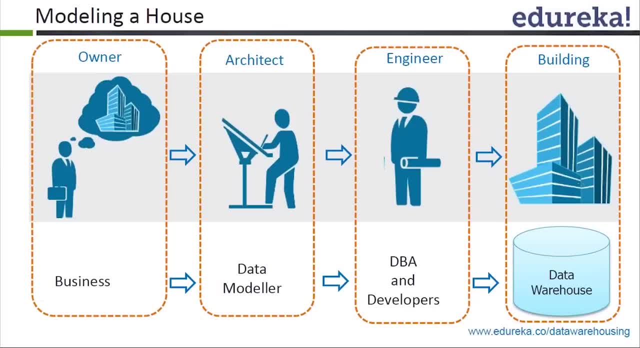 So what exactly this situation says is that if he would have built a mall, maybe he would have seen the proper exit strategy for his mall. So what exactly this situation says is that if he would have built a mall, maybe he would have seen the proper exit strategy for his mall. 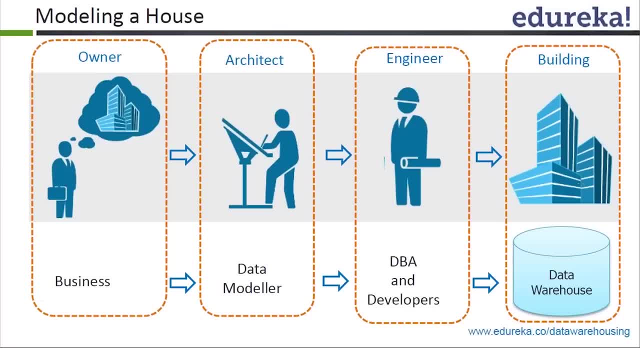 So what exactly this situation says is that if he would have built a mall, maybe he would have seen the proper exit strategy for his mall. So what exactly this situation says is that if he would have built a mall, maybe he would have seen the proper exit strategy for his mall. 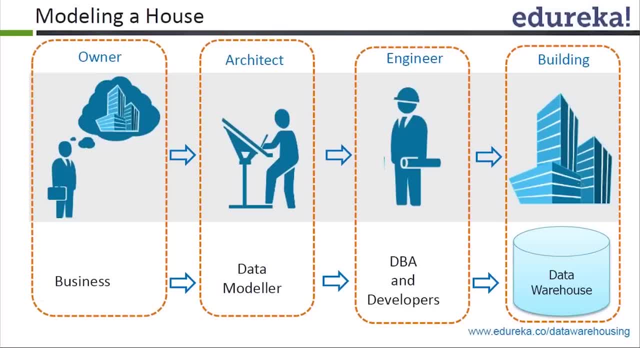 So what exactly this situation says is that if he would have built a mall, maybe he would have seen the proper exit strategy for his mall. So what exactly this situation says is that if he would have built a mall, maybe he would have seen the proper exit strategy for his mall. 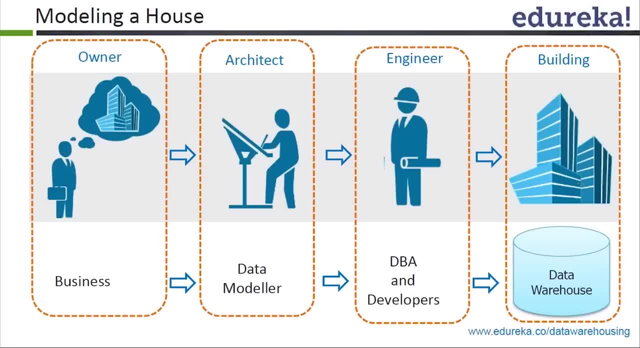 So what exactly this situation says is that if he would have built a mall, maybe he would have seen the proper exit strategy for his mall. So what exactly this situation says is that if he would have built a mall, maybe he would have seen the proper exit strategy for his mall. 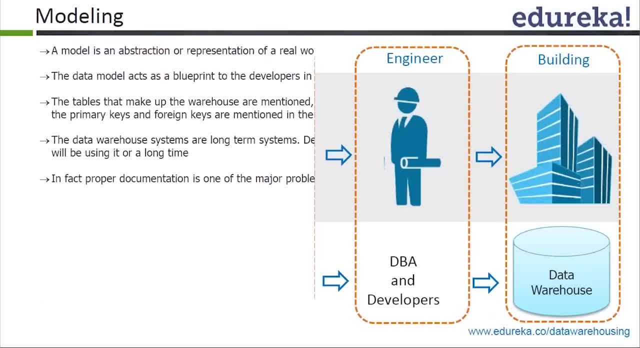 So what exactly this situation says is that if he would have built a mall, maybe he would have seen the proper exit strategy for his mall. So what exactly this situation says is that if he would have built a mall, maybe he would have seen the proper exit strategy for his mall. 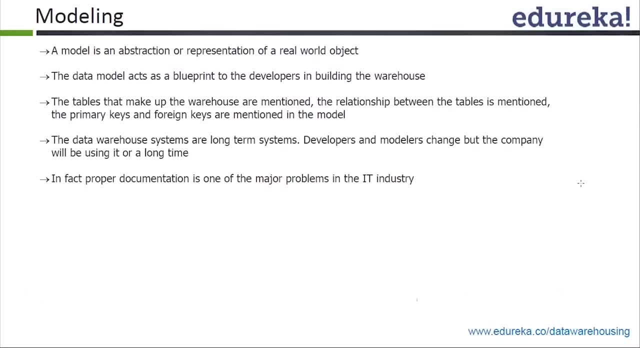 So what exactly this situation says is that if he would have built a mall, maybe he would have seen the proper exit strategy for his mall. So what exactly this situation says is that if he would have built a mall, maybe he would have seen the proper exit strategy for his mall. 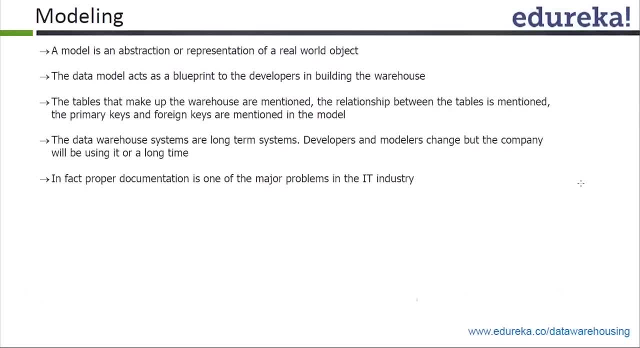 So what exactly this situation says is that if he would have built a mall, maybe he would have seen the proper exit strategy for his mall. So what exactly this situation says is that if he would have built a mall, maybe he would have seen the proper exit strategy for his mall. 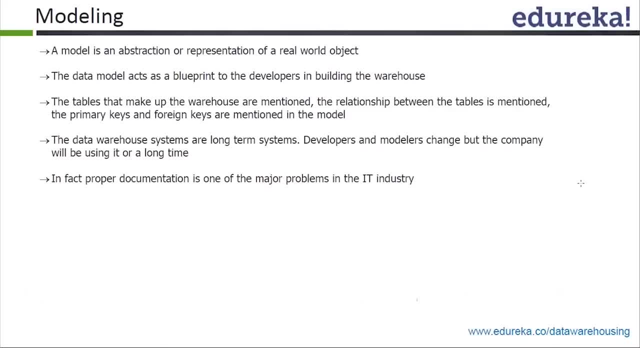 So what exactly this situation says is that if he would have built a mall, maybe he would have seen the proper exit strategy for his mall. So what exactly this situation says is that if he would have built a mall, maybe he would have seen the proper exit strategy for his mall. 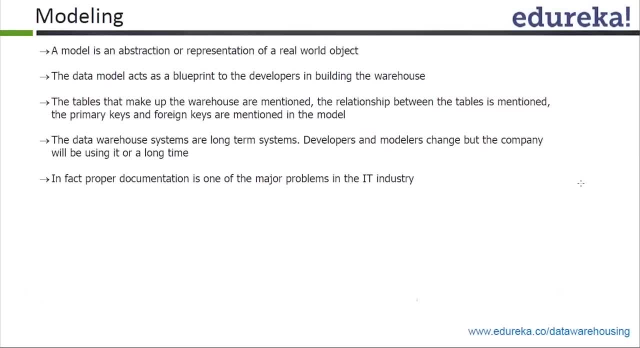 So what exactly this situation says is that if he would have built a mall, maybe he would have seen the proper exit strategy for his mall. So what exactly this situation says is that if he would have built a mall, maybe he would have seen the proper exit strategy for his mall. 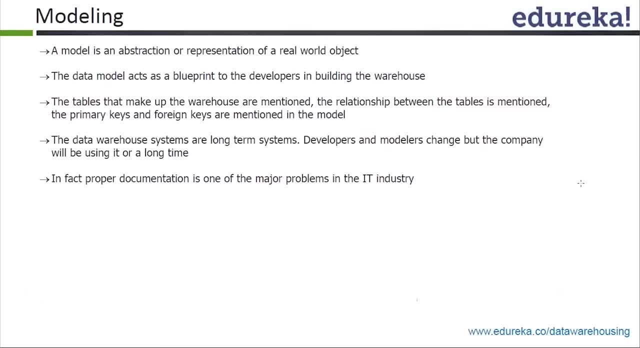 So what exactly this situation says is that if he would have built a mall, maybe he would have seen the proper exit strategy for his mall. So what exactly this situation says is that if he would have built a mall, maybe he would have seen the proper exit strategy for his mall. 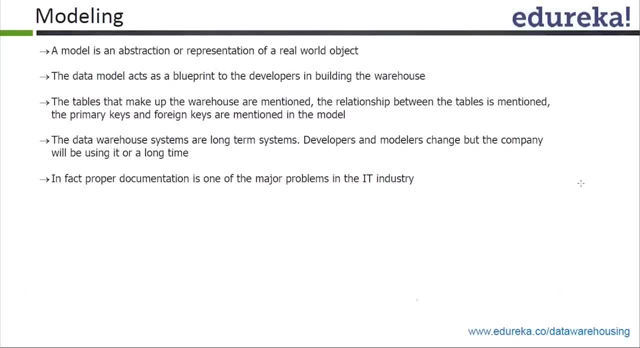 So what exactly this situation says is that if he would have built a mall, maybe he would have seen the proper exit strategy for his mall. So what exactly this situation says is that if he would have built a mall, maybe he would have seen the proper exit strategy for his mall. 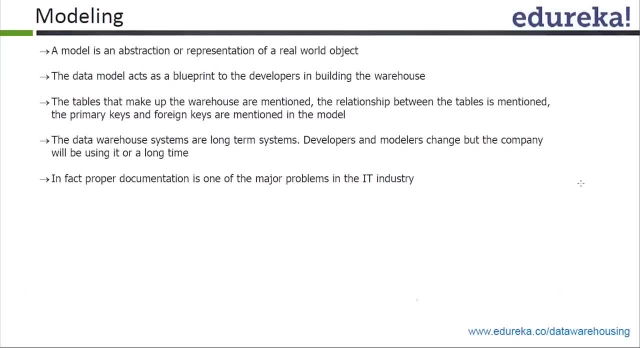 So what exactly this situation says is that if he would have built a mall, maybe he would have seen the proper exit strategy for his mall. So what exactly this situation says is that if he would have built a mall, maybe he would have seen the proper exit strategy for his mall. 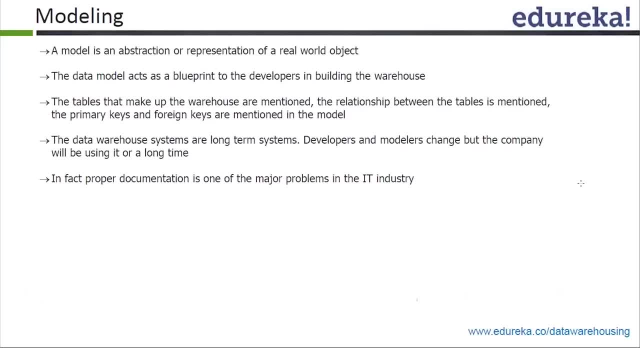 So what exactly this situation says is that if he would have built a mall, maybe he would have seen the proper exit strategy for his mall. So what exactly this situation says is that if he would have built a mall, maybe he would have seen the proper exit strategy for his mall. 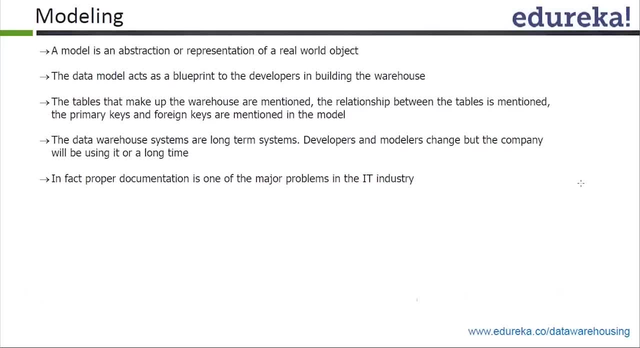 So what exactly this situation says is that if he would have built a mall, maybe he would have seen the proper exit strategy for his mall. So what exactly this situation says is that if he would have built a mall, maybe he would have seen the proper exit strategy for his mall. 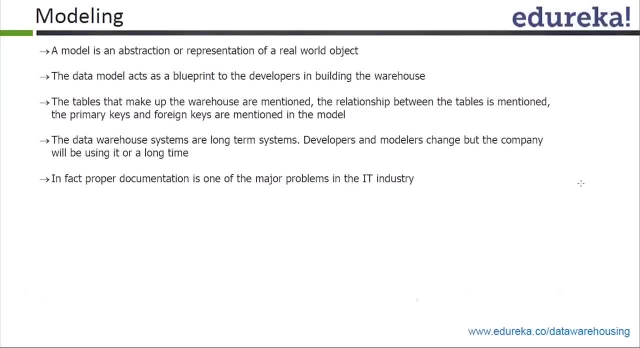 So what exactly this situation says is that if he would have built a mall, maybe he would have seen the proper exit strategy for his mall. So what exactly this situation says is that if he would have built a mall, maybe he would have seen the proper exit strategy for his mall. 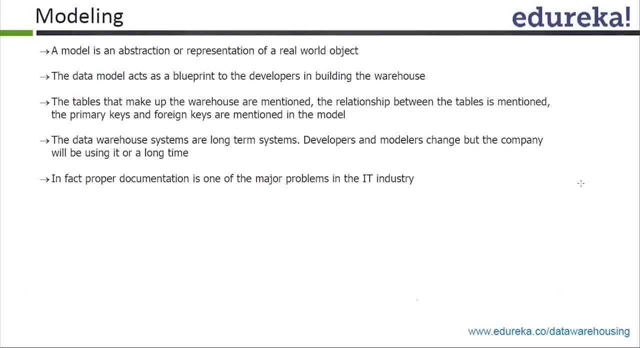 So what exactly this situation says is that if he would have built a mall, maybe he would have seen the proper exit strategy for his mall. So what exactly this situation says is that if he would have built a mall, maybe he would have seen the proper exit strategy for his mall. 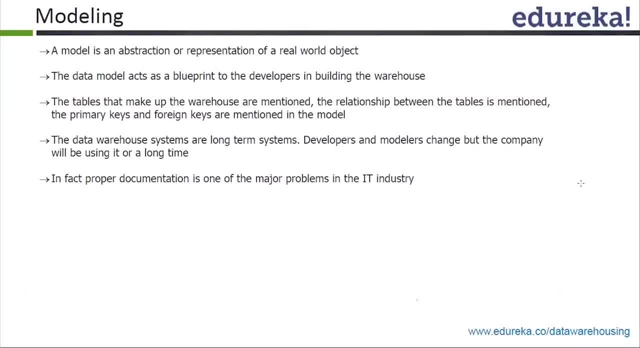 So what exactly this situation says is that if he would have built a mall, maybe he would have seen the proper exit strategy for his mall. So what exactly this situation says is that if he would have built a mall, maybe he would have seen the proper exit strategy for his mall. 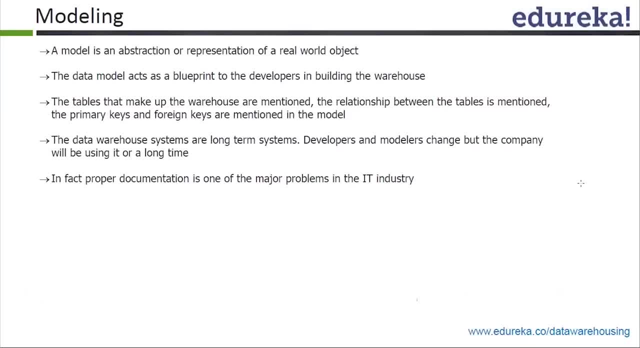 So what exactly this situation says is that if he would have built a mall, maybe he would have seen the proper exit strategy for his mall. So what exactly this situation says is that if he would have built a mall, maybe he would have seen the proper exit strategy for his mall. 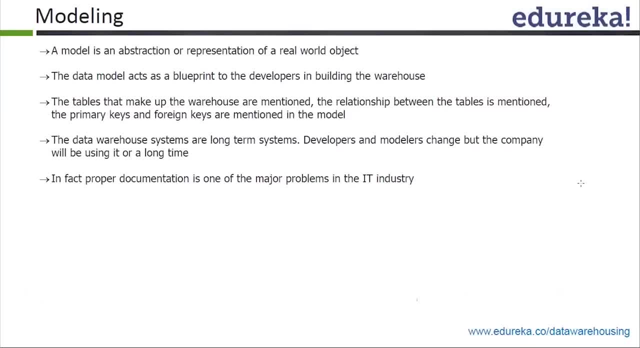 So what exactly this situation says is that if he would have built a mall, maybe he would have seen the proper exit strategy for his mall. So what exactly this situation says is that if he would have built a mall, maybe he would have seen the proper exit strategy for his mall. 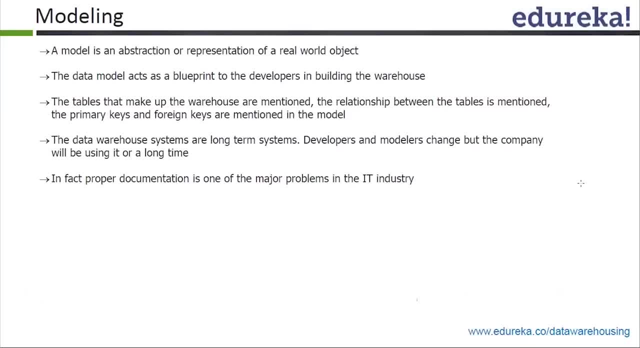 So what exactly this situation says is that if he would have built a mall, maybe he would have seen the proper exit strategy for his mall. So what exactly this situation says is that if he would have built a mall, maybe he would have seen the proper exit strategy for his mall. 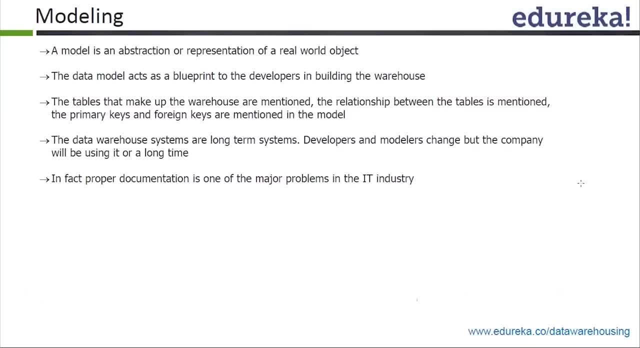 So what exactly this situation says is that if he would have built a mall, maybe he would have seen the proper exit strategy for his mall. So what exactly this situation says is that if he would have built a mall, maybe he would have seen the proper exit strategy for his mall. 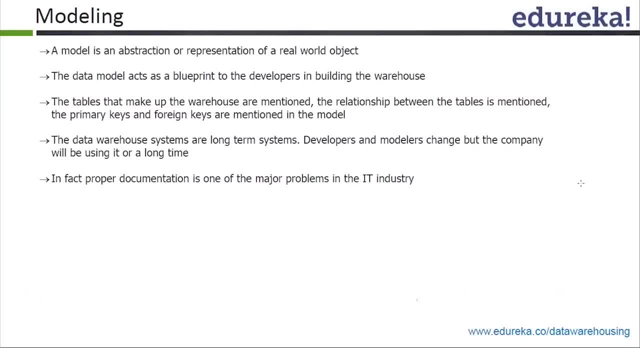 So what exactly this situation says is that if he would have built a mall, maybe he would have seen the proper exit strategy for his mall. So what exactly this situation says is that if he would have built a mall, maybe he would have seen the proper exit strategy for his mall. 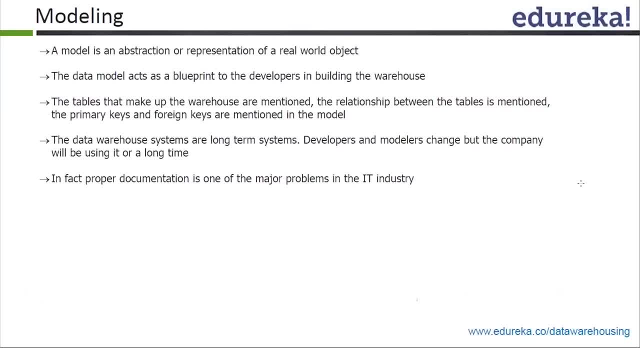 So what exactly this situation says is that if he would have built a mall, maybe he would have seen the proper exit strategy for his mall. So what exactly this situation says is that if he would have built a mall, maybe he would have seen the proper exit strategy for his mall. 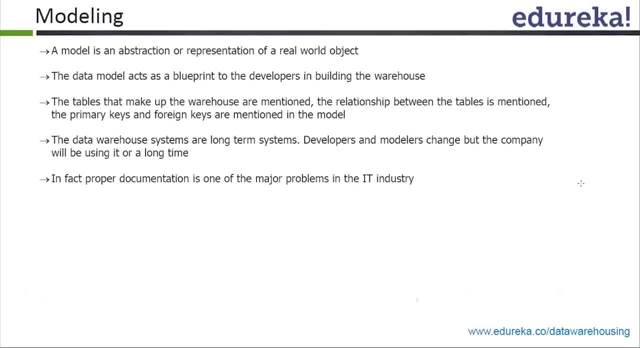 So what exactly this situation says is that if he would have built a mall, maybe he would have seen the proper exit strategy for his mall. So what exactly this situation says is that if he would have built a mall, maybe he would have seen the proper exit strategy for his mall. 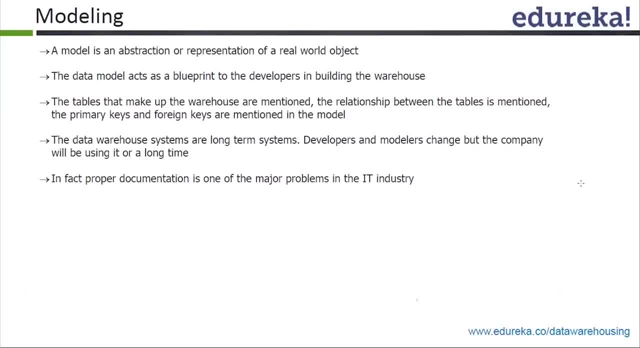 So what exactly this situation says is that if he would have built a mall, maybe he would have seen the proper exit strategy for his mall. So what exactly this situation says is that if he would have built a mall, maybe he would have seen the proper exit strategy for his mall. 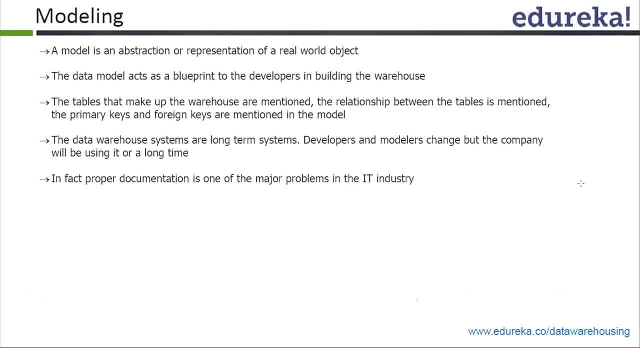 So what exactly this situation says is that if he would have built a mall, maybe he would have seen the proper exit strategy for his mall. So what exactly this situation says is that if he would have built a mall, maybe he would have seen the proper exit strategy for his mall. 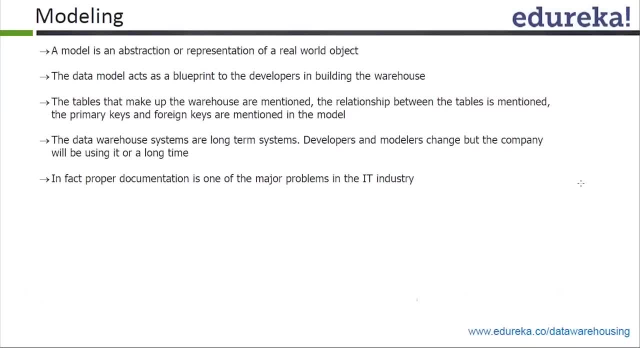 So what exactly this situation says is that if he would have built a mall, maybe he would have seen the proper exit strategy for his mall. So what exactly this situation says is that if he would have built a mall, maybe he would have seen the proper exit strategy for his mall. 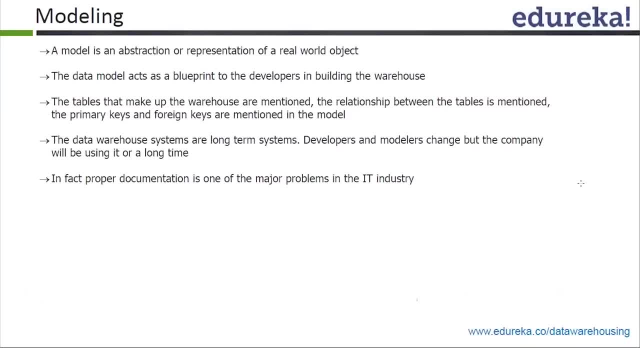 So what exactly this situation says is that if he would have built a mall, maybe he would have seen the proper exit strategy for his mall. So what exactly this situation says is that if he would have built a mall, maybe he would have seen the proper exit strategy for his mall. 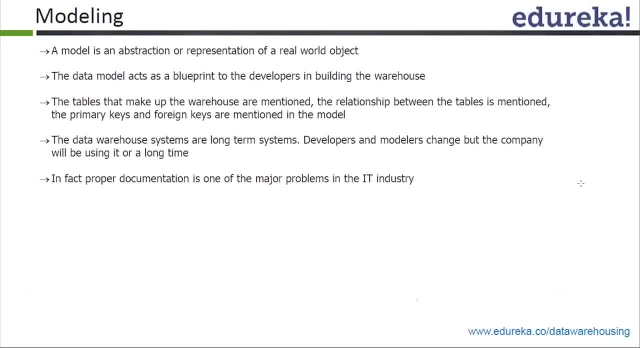 So what exactly this situation says is that if he would have built a mall, maybe he would have seen the proper exit strategy for his mall. So what exactly this situation says is that if he would have built a mall, maybe he would have seen the proper exit strategy for his mall. 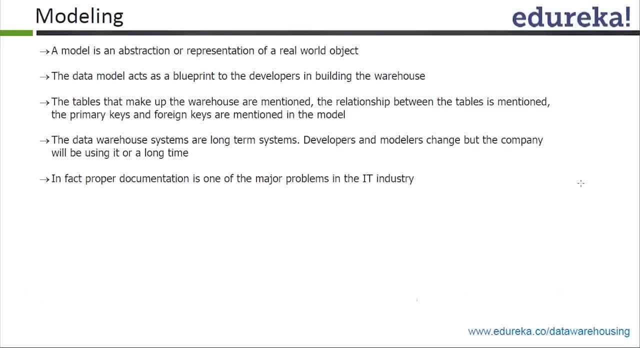 So what exactly this situation says is that if he would have built a mall, maybe he would have seen the proper exit strategy for his mall. So what exactly this situation says is that if he would have built a mall, maybe he would have seen the proper exit strategy for his mall. 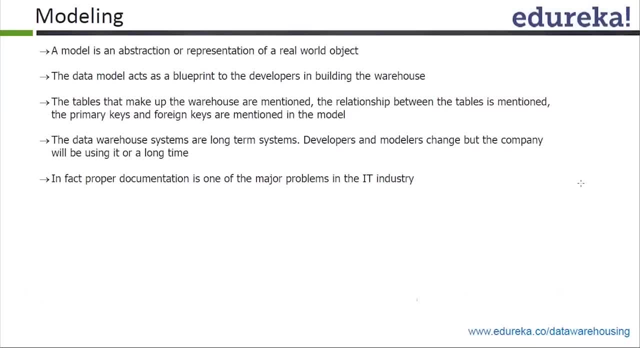 So what exactly this situation says is that if he would have built a mall, maybe he would have seen the proper exit strategy for his mall. So what exactly this situation says is that if he would have built a mall, maybe he would have seen the proper exit strategy for his mall. 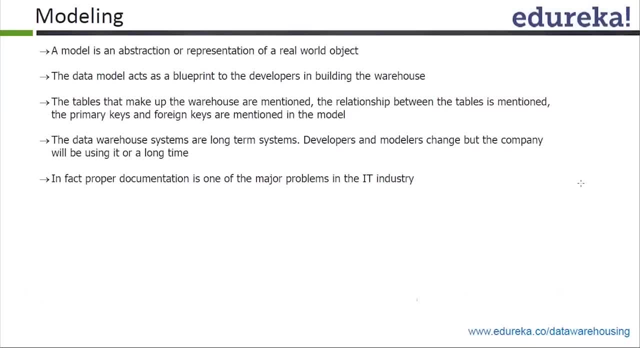 So what exactly this situation says is that if he would have built a mall, maybe he would have seen the proper exit strategy for his mall. So what exactly this situation says is that if he would have built a mall, maybe he would have seen the proper exit strategy for his mall. 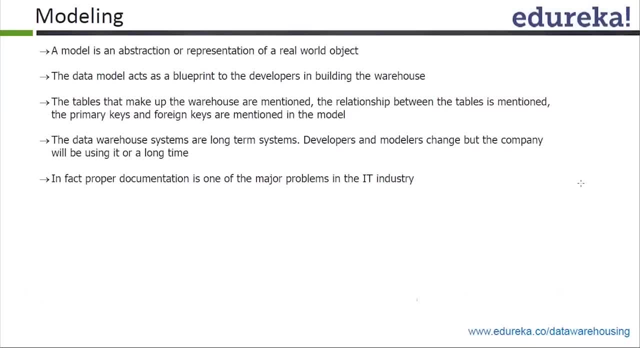 So what exactly this situation says is that if he would have built a mall, maybe he would have seen the proper exit strategy for his mall. So what exactly this situation says is that if he would have built a mall, maybe he would have seen the proper exit strategy for his mall. 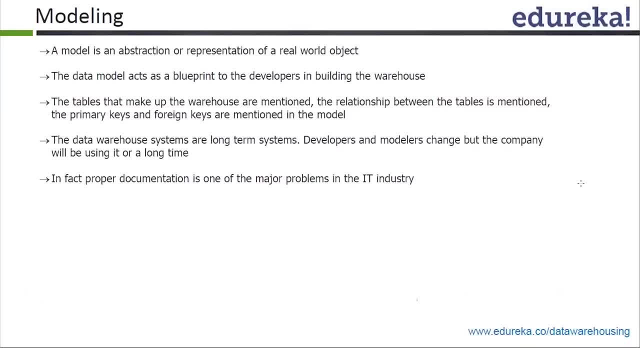 So what exactly this situation says is that if he would have built a mall, maybe he would have seen the proper exit strategy for his mall. So what exactly this situation says is that if he would have built a mall, maybe he would have seen the proper exit strategy for his mall. 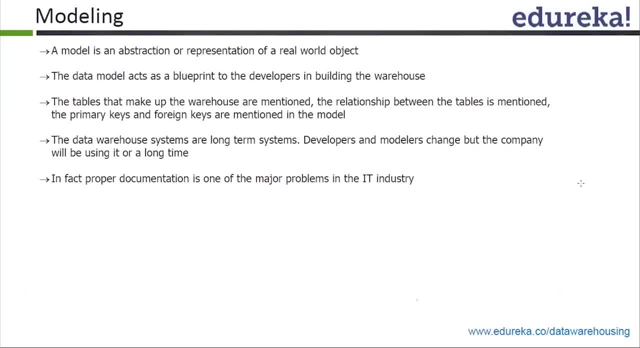 So what exactly this situation says is that if he would have built a mall, maybe he would have seen the proper exit strategy for his mall. So what exactly this situation says is that if he would have built a mall, maybe he would have seen the proper exit strategy for his mall. 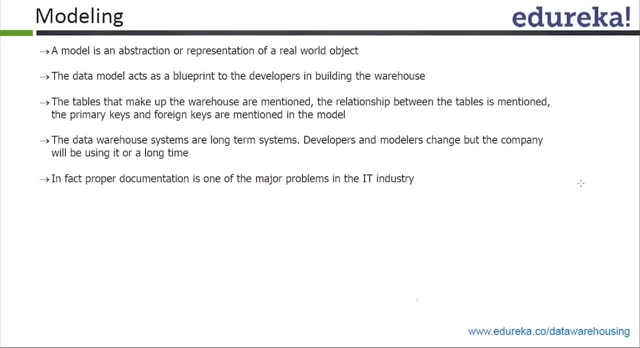 So what exactly this situation says is that if he would have built a mall, maybe he would have seen the proper exit strategy for his mall. So what exactly this situation says is that if he would have built a mall, maybe he would have seen the proper exit strategy for his mall. 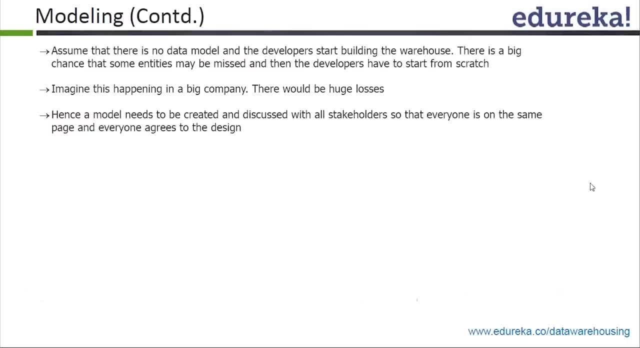 So what exactly this situation says is that if he would have built a mall, maybe he would have seen the proper exit strategy for his mall. So what exactly this situation says is that if he would have built a mall, maybe he would have seen the proper exit strategy for his mall. 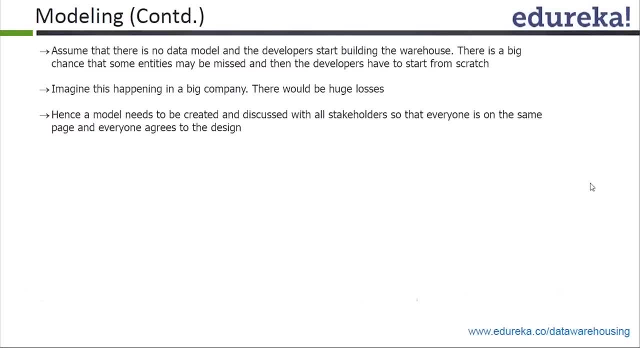 So what exactly this situation says is that if he would have built a mall, maybe he would have seen the proper exit strategy for his mall. So what exactly this situation says is that if he would have built a mall, maybe he would have seen the proper exit strategy for his mall. 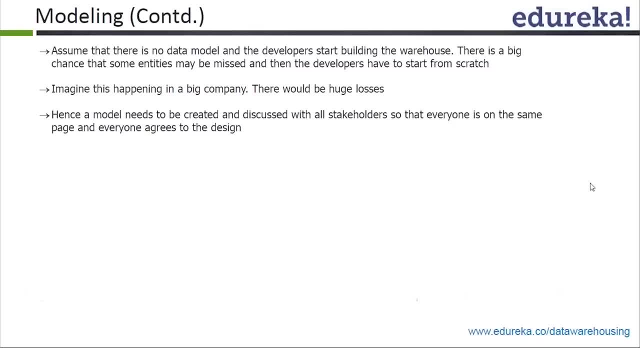 So what exactly this situation says is that if he would have built a mall, maybe he would have seen the proper exit strategy for his mall. So what exactly this situation says is that if he would have built a mall, maybe he would have seen the proper exit strategy for his mall. 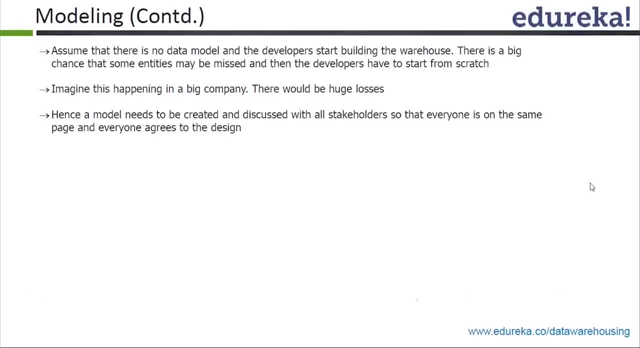 So what exactly this situation says is that if he would have built a mall, maybe he would have seen the proper exit strategy for his mall. So what exactly this situation says is that if he would have built a mall, maybe he would have seen the proper exit strategy for his mall. 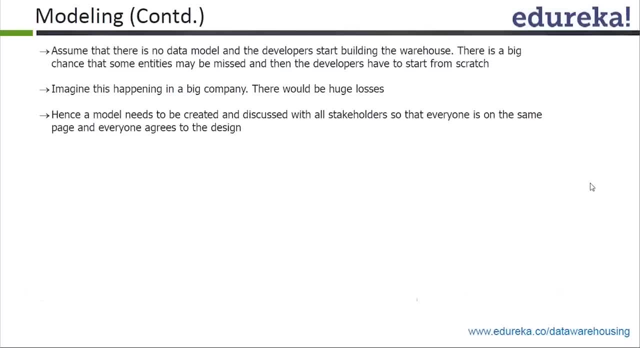 So what exactly this situation says is that if he would have built a mall, maybe he would have seen the proper exit strategy for his mall. So what exactly this situation says is that if he would have built a mall, maybe he would have seen the proper exit strategy for his mall. 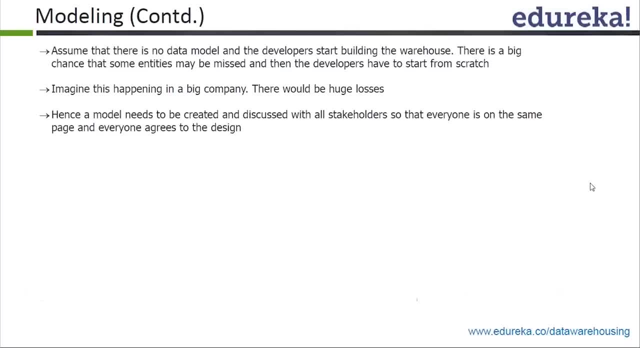 So what exactly this situation says is that if he would have built a mall, maybe he would have seen the proper exit strategy for his mall. So what exactly this situation says is that if he would have built a mall, maybe he would have seen the proper exit strategy for his mall. 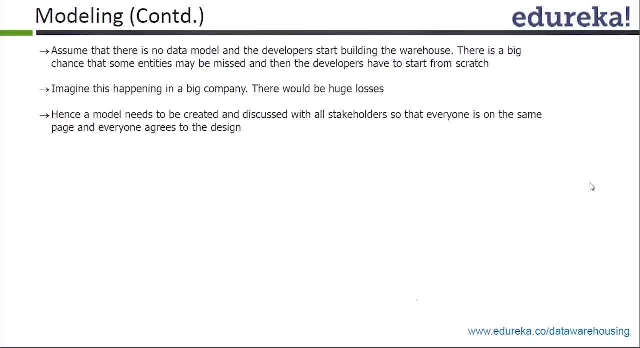 So what exactly this situation says is that if he would have built a mall, maybe he would have seen the proper exit strategy for his mall. So what exactly this situation says is that if he would have built a mall, maybe he would have seen the proper exit strategy for his mall. 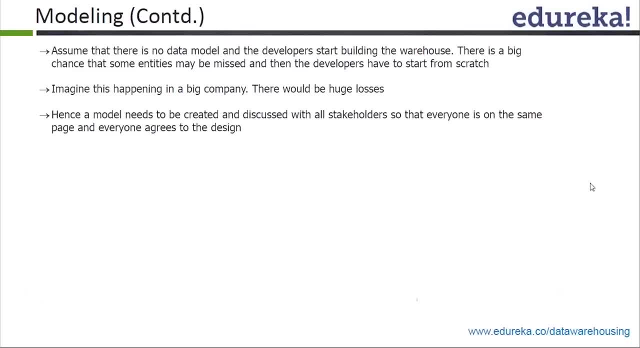 So what exactly this situation says is that if he would have built a mall, maybe he would have seen the proper exit strategy for his mall. So what exactly this situation says is that if he would have built a mall, maybe he would have seen the proper exit strategy for his mall. 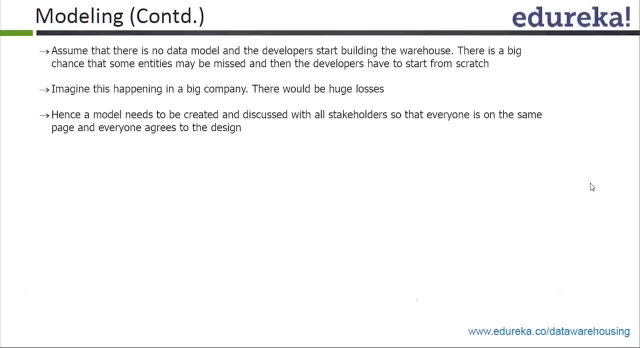 So what exactly this situation says is that if he would have built a mall, maybe he would have seen the proper exit strategy for his mall. So what exactly this situation says is that if he would have built a mall, maybe he would have seen the proper exit strategy for his mall. 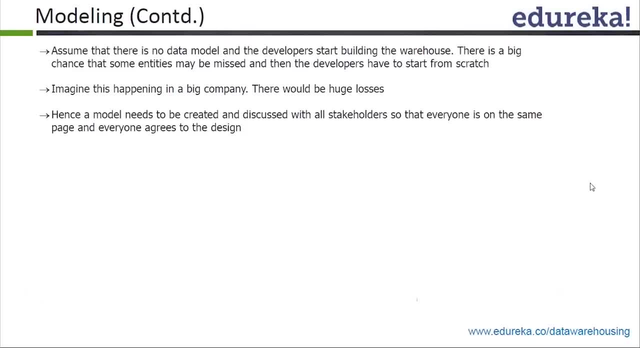 So what exactly this situation says is that if he would have built a mall, maybe he would have seen the proper exit strategy for his mall. So what exactly this situation says is that if he would have built a mall, maybe he would have seen the proper exit strategy for his mall. 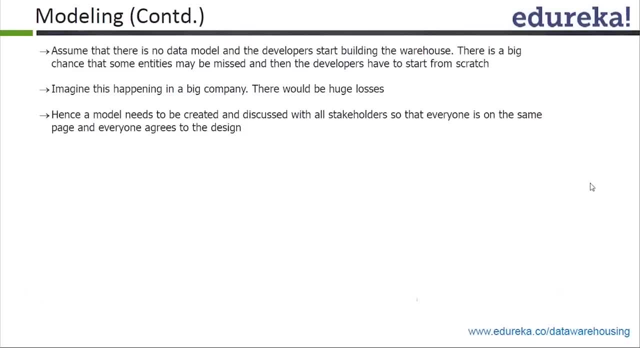 So what exactly this situation says is that if he would have built a mall, maybe he would have seen the proper exit strategy for his mall. So what exactly this situation says is that if he would have built a mall, maybe he would have seen the proper exit strategy for his mall. 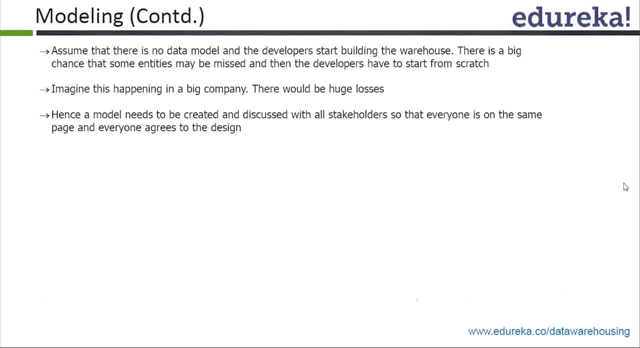 So what exactly this situation says is that if he would have built a mall, maybe he would have seen the proper exit strategy for his mall. So what exactly this situation says is that if he would have built a mall, maybe he would have seen the proper exit strategy for his mall. 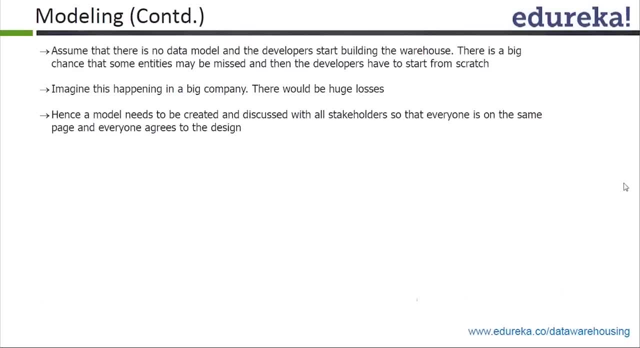 So what exactly this situation says is that if he would have built a mall, maybe he would have seen the proper exit strategy for his mall. So what exactly this situation says is that if he would have built a mall, maybe he would have seen the proper exit strategy for his mall. 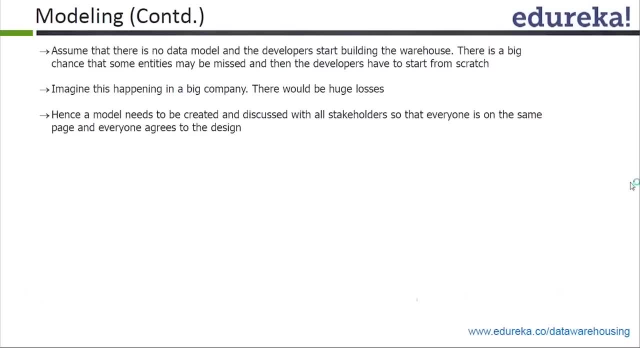 So what exactly this situation says is that if he would have built a mall, maybe he would have seen the proper exit strategy for his mall. So what exactly this situation says is that if he would have built a mall, maybe he would have seen the proper exit strategy for his mall. 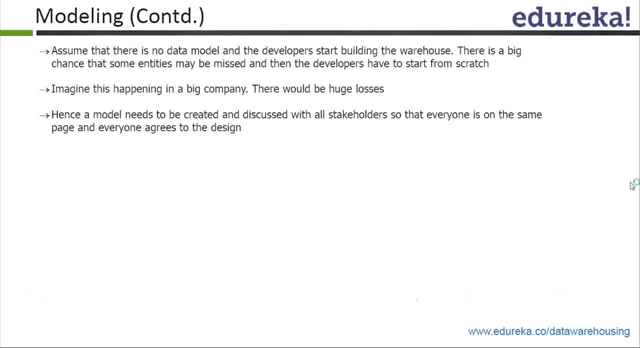 So what exactly this situation says is that if he would have built a mall, maybe he would have seen the proper exit strategy for his mall. So what exactly this situation says is that if he would have built a mall, maybe he would have seen the proper exit strategy for his mall. 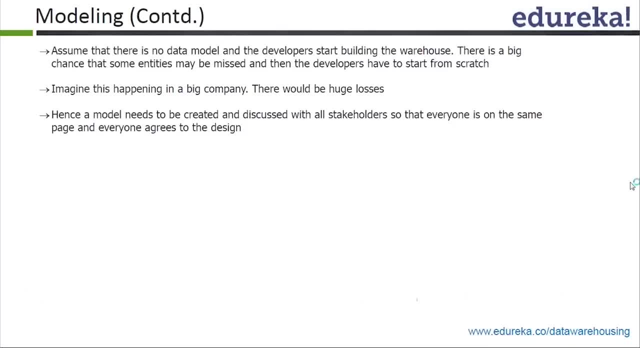 So what exactly this situation says is that if he would have built a mall, maybe he would have seen the proper exit strategy for his mall. So what exactly this situation says is that if he would have built a mall, maybe he would have seen the proper exit strategy for his mall. 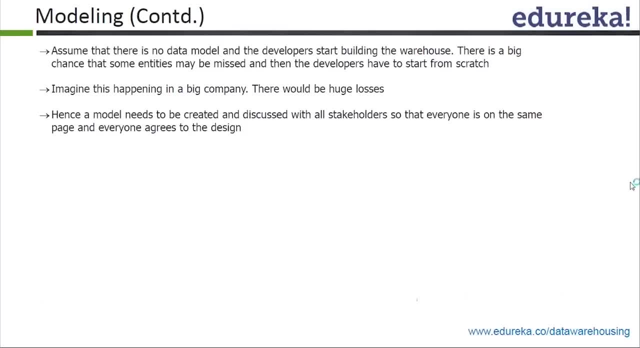 So what exactly this situation says is that if he would have built a mall, maybe he would have seen the proper exit strategy for his mall. So what exactly this situation says is that if he would have built a mall, maybe he would have seen the proper exit strategy for his mall. 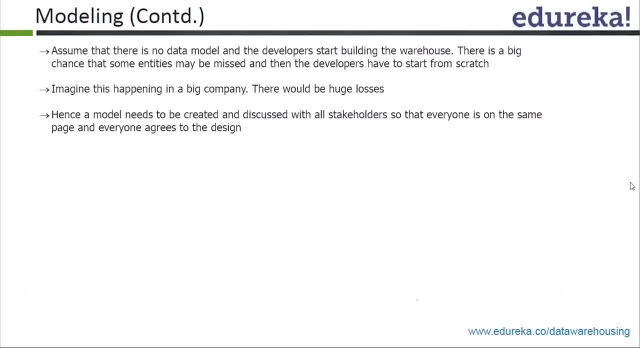 So what exactly this situation says is that if he would have built a mall, maybe he would have seen the proper exit strategy for his mall. So what exactly this situation says is that if he would have built a mall, maybe he would have seen the proper exit strategy for his mall. 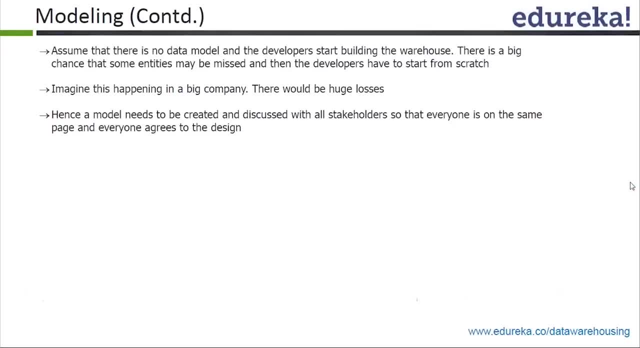 So what exactly this situation says is that if he would have built a mall, maybe he would have seen the proper exit strategy for his mall. So what exactly this situation says is that if he would have built a mall, maybe he would have seen the proper exit strategy for his mall. 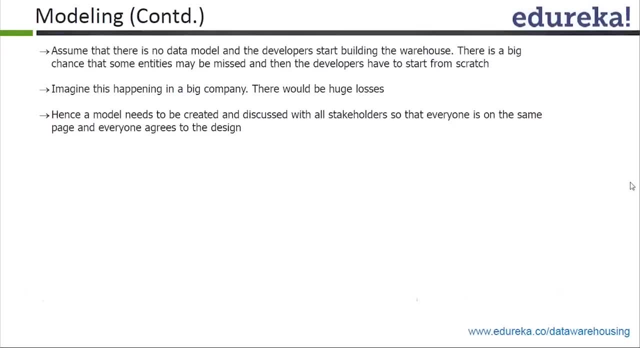 So what exactly this situation says is that if he would have built a mall, maybe he would have seen the proper exit strategy for his mall. So what exactly this situation says is that if he would have built a mall, maybe he would have seen the proper exit strategy for his mall. 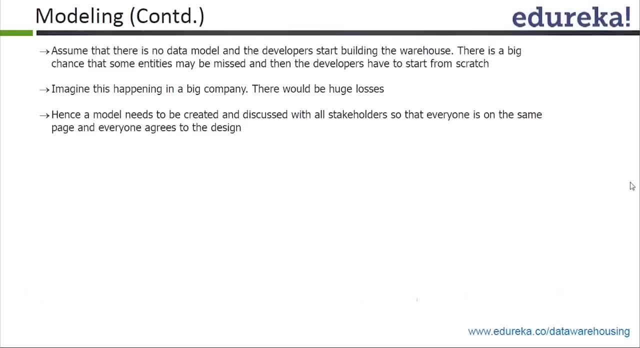 So what exactly this situation says is that if he would have built a mall, maybe he would have seen the proper exit strategy for his mall. So what exactly this situation says is that if he would have built a mall, maybe he would have seen the proper exit strategy for his mall. 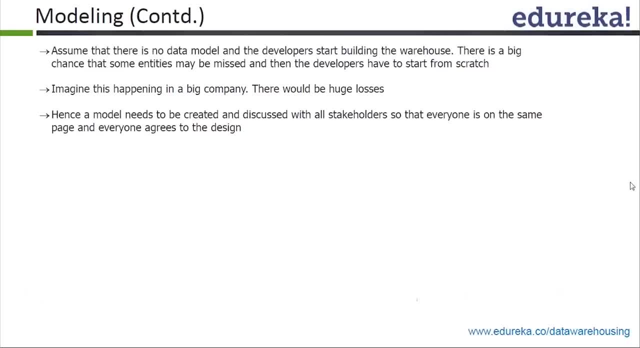 So what exactly this situation says is that if he would have built a mall, maybe he would have seen the proper exit strategy for his mall. So what exactly this situation says is that if he would have built a mall, maybe he would have seen the proper exit strategy for his mall. 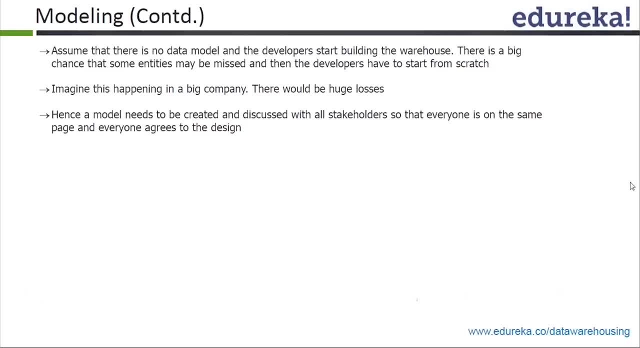 So what exactly this situation says is that if he would have built a mall, maybe he would have seen the proper exit strategy for his mall. So what exactly this situation says is that if he would have built a mall, maybe he would have seen the proper exit strategy for his mall. 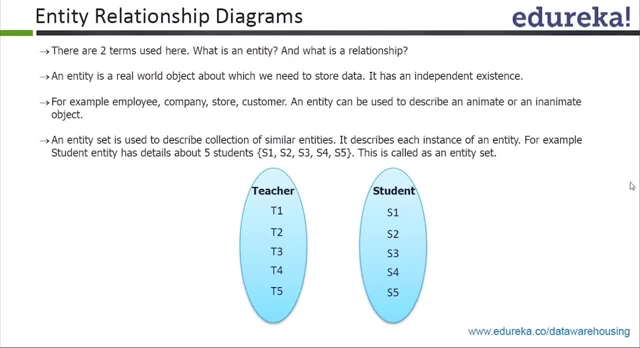 So what exactly this situation says is that if he would have built a mall, maybe he would have seen the proper exit strategy for his mall. So what exactly this situation says is that if he would have built a mall, maybe he would have seen the proper exit strategy for his mall. 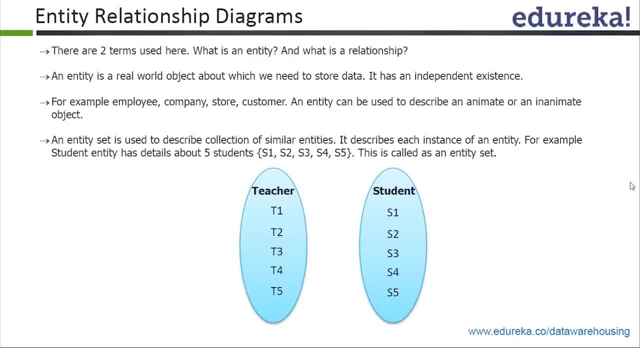 So what exactly this situation says is that if he would have built a mall, maybe he would have seen the proper exit strategy for his mall. So what exactly this situation says is that if he would have built a mall, maybe he would have seen the proper exit strategy for his mall. 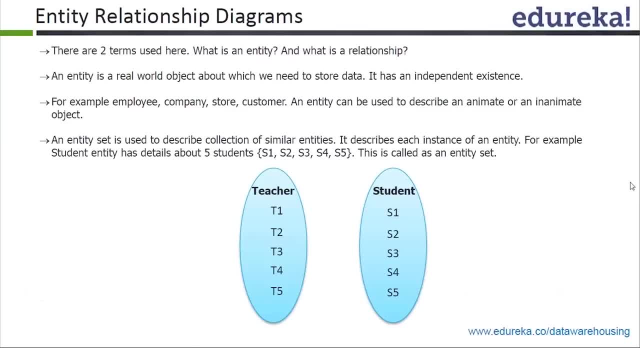 So what exactly this situation says is that if he would have built a mall, maybe he would have seen the proper exit strategy for his mall. So what exactly this situation says is that if he would have built a mall, maybe he would have seen the proper exit strategy for his mall. 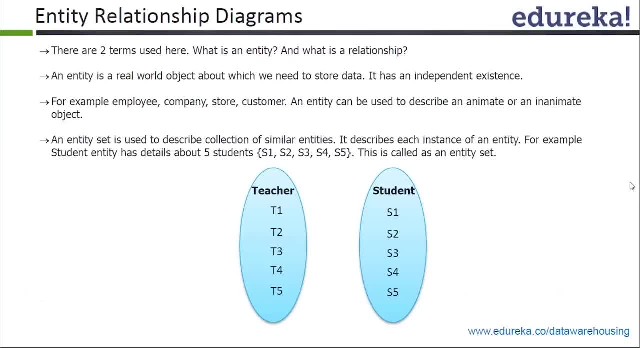 So what exactly this situation says is that if he would have built a mall, maybe he would have seen the proper exit strategy for his mall. So what exactly this situation says is that if he would have built a mall, maybe he would have seen the proper exit strategy for his mall. 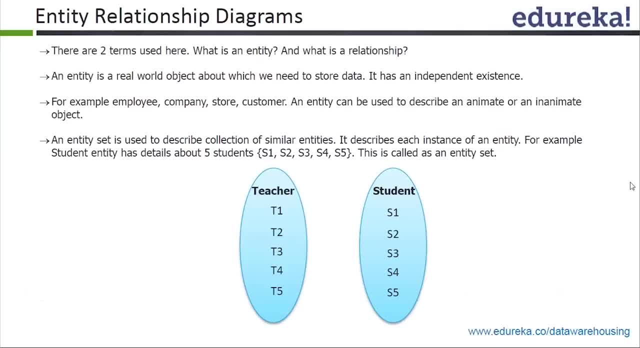 So what exactly this situation says is that if he would have built a mall, maybe he would have seen the proper exit strategy for his mall. So what exactly this situation says is that if he would have built a mall, maybe he would have seen the proper exit strategy for his mall. 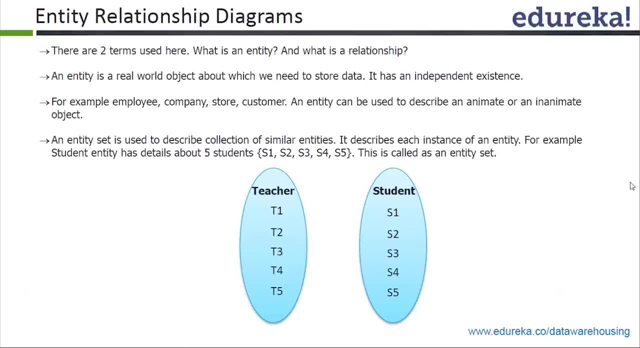 So what exactly this situation says is that if he would have built a mall, maybe he would have seen the proper exit strategy for his mall. So what exactly this situation says is that if he would have built a mall, maybe he would have seen the proper exit strategy for his mall. 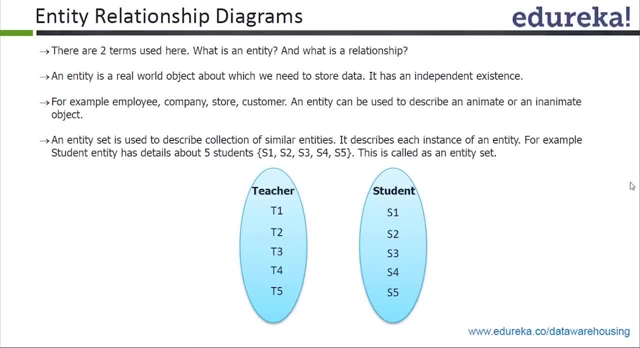 So what exactly this situation says is that if he would have built a mall, maybe he would have seen the proper exit strategy for his mall. So what exactly this situation says is that if he would have built a mall, maybe he would have seen the proper exit strategy for his mall. 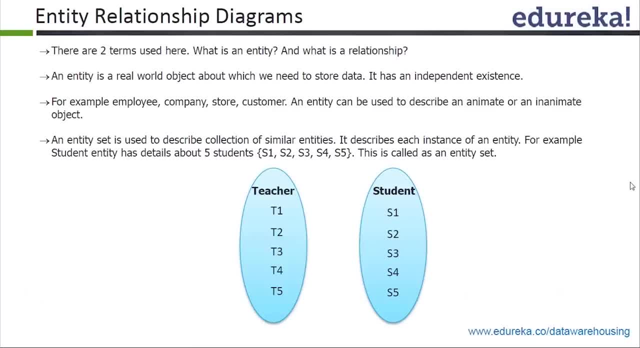 So what exactly this situation says is that if he would have built a mall, maybe he would have seen the proper exit strategy for his mall. So what exactly this situation says is that if he would have built a mall, maybe he would have seen the proper exit strategy for his mall. 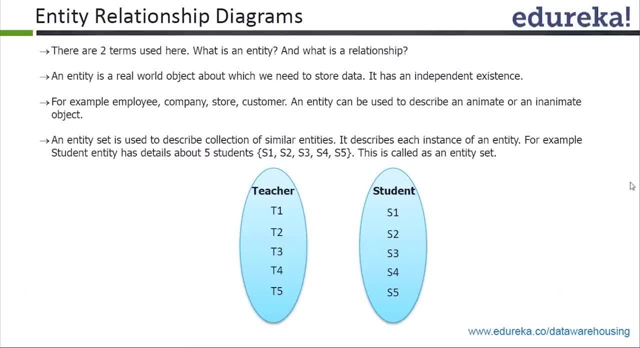 So what exactly this situation says is that if he would have built a mall, maybe he would have seen the proper exit strategy for his mall. So what exactly this situation says is that if he would have built a mall, maybe he would have seen the proper exit strategy for his mall. 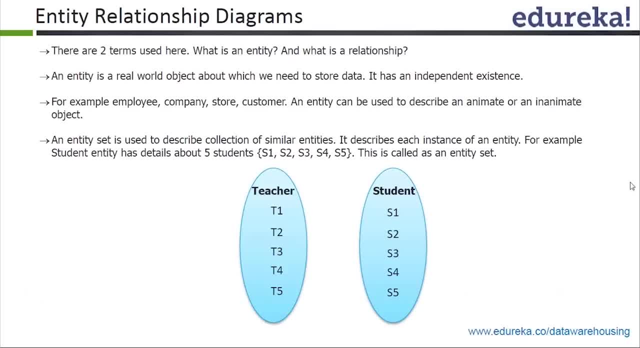 So what exactly this situation says is that if he would have built a mall, maybe he would have seen the proper exit strategy for his mall. So what exactly this situation says is that if he would have built a mall, maybe he would have seen the proper exit strategy for his mall. 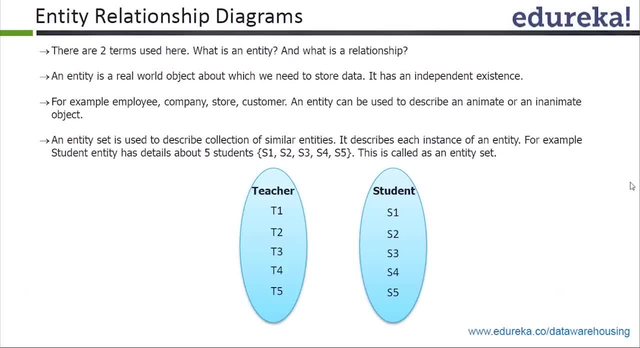 So what exactly this situation says is that if he would have built a mall, maybe he would have seen the proper exit strategy for his mall. So what exactly this situation says is that if he would have built a mall, maybe he would have seen the proper exit strategy for his mall. 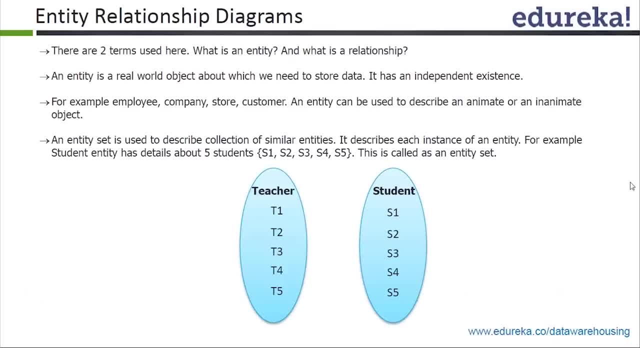 So what exactly this situation says is that if he would have built a mall, maybe he would have seen the proper exit strategy for his mall. So what exactly this situation says is that if he would have built a mall, maybe he would have seen the proper exit strategy for his mall. 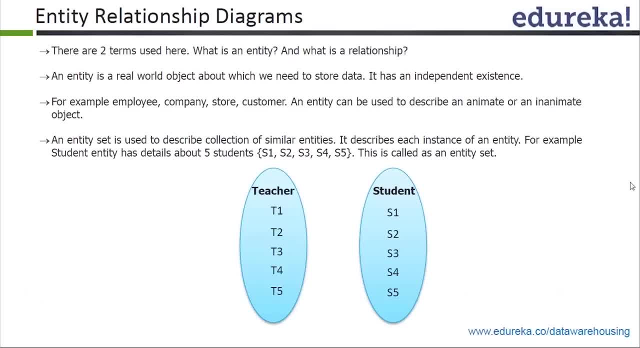 So what exactly this situation says is that if he would have built a mall, maybe he would have seen the proper exit strategy for his mall. So what exactly this situation says is that if he would have built a mall, maybe he would have seen the proper exit strategy for his mall. 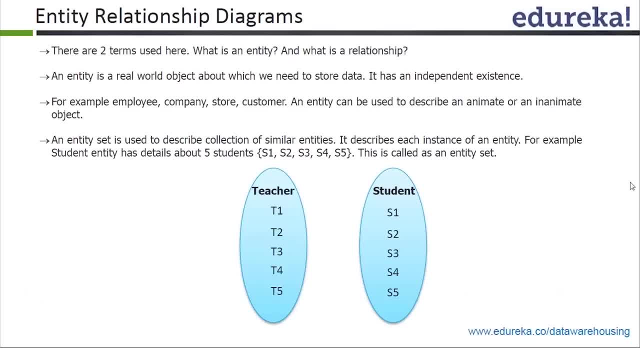 So what exactly this situation says is that if he would have built a mall, maybe he would have seen the proper exit strategy for his mall. So what exactly this situation says is that if he would have built a mall, maybe he would have seen the proper exit strategy for his mall. 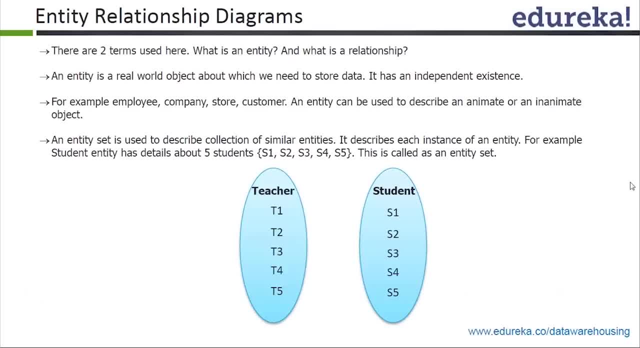 So what exactly this situation says is that if he would have built a mall, maybe he would have seen the proper exit strategy for his mall. So what exactly this situation says is that if he would have built a mall, maybe he would have seen the proper exit strategy for his mall. 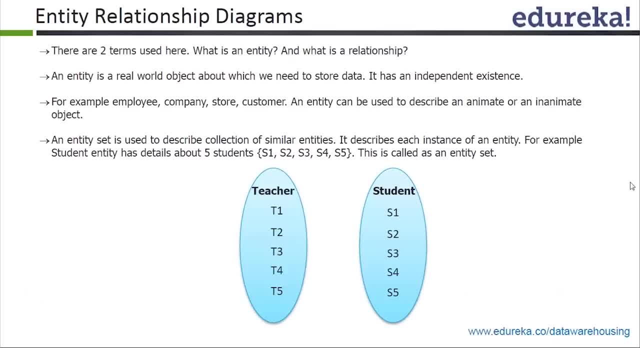 So what exactly this situation says is that if he would have built a mall, maybe he would have seen the proper exit strategy for his mall. So what exactly this situation says is that if he would have built a mall, maybe he would have seen the proper exit strategy for his mall. 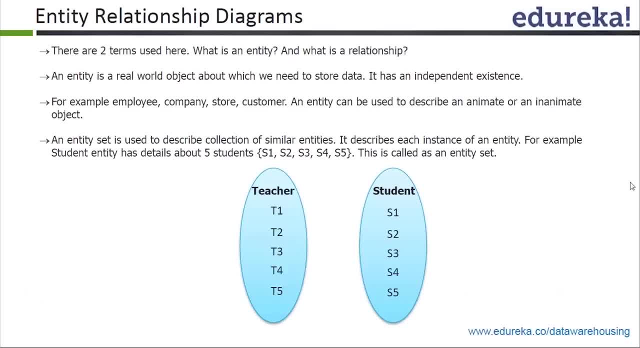 So what exactly this situation says is that if he would have built a mall, maybe he would have seen the proper exit strategy for his mall. So what exactly this situation says is that if he would have built a mall, maybe he would have seen the proper exit strategy for his mall. 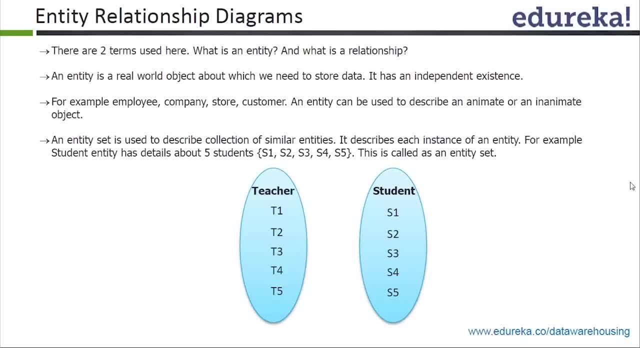 So what exactly this situation says is that if he would have built a mall, maybe he would have seen the proper exit strategy for his mall. So what exactly this situation says is that if he would have built a mall, maybe he would have seen the proper exit strategy for his mall. 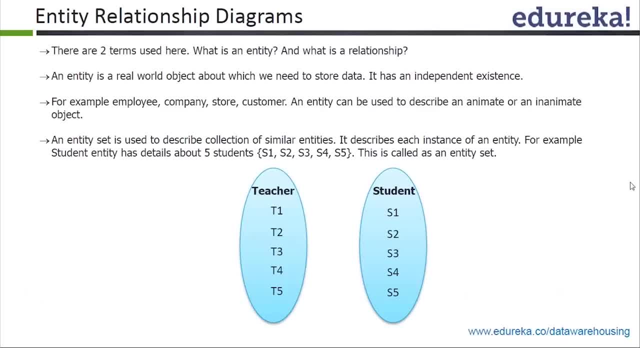 So what exactly this situation says is that if he would have built a mall, maybe he would have seen the proper exit strategy for his mall. So what exactly this situation says is that if he would have built a mall, maybe he would have seen the proper exit strategy for his mall. 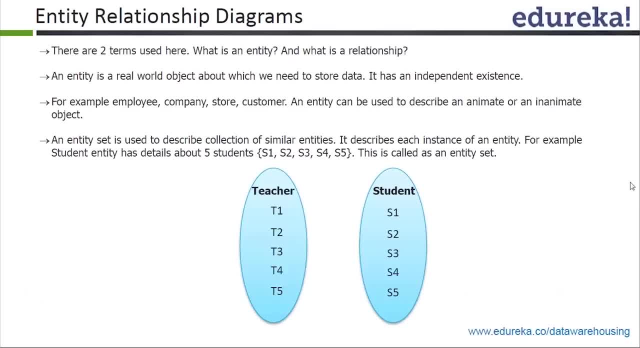 So what exactly this situation says is that if he would have built a mall, maybe he would have seen the proper exit strategy for his mall. So what exactly this situation says is that if he would have built a mall, maybe he would have seen the proper exit strategy for his mall. 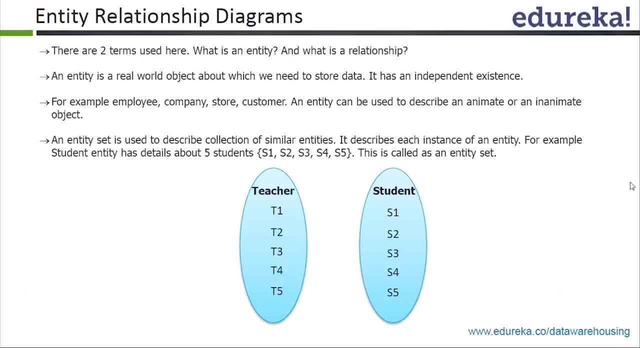 So what exactly this situation says is that if he would have built a mall, maybe he would have seen the proper exit strategy for his mall. So what exactly this situation says is that if he would have built a mall, maybe he would have seen the proper exit strategy for his mall. 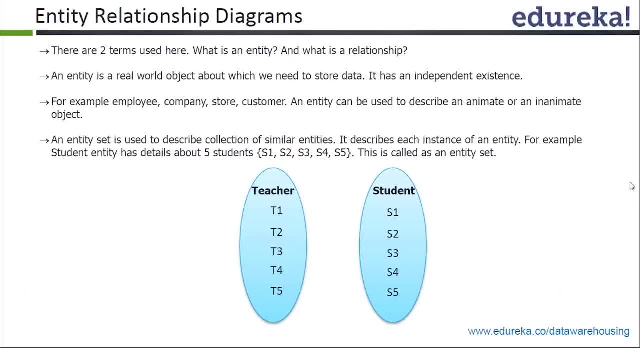 So what exactly this situation says is that if he would have built a mall, maybe he would have seen the proper exit strategy for his mall. So what exactly this situation says is that if he would have built a mall, maybe he would have seen the proper exit strategy for his mall. 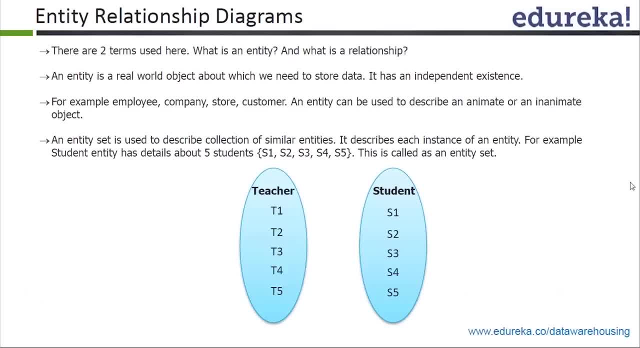 So what exactly this situation says is that if he would have built a mall, maybe he would have seen the proper exit strategy for his mall. So what exactly this situation says is that if he would have built a mall, maybe he would have seen the proper exit strategy for his mall. 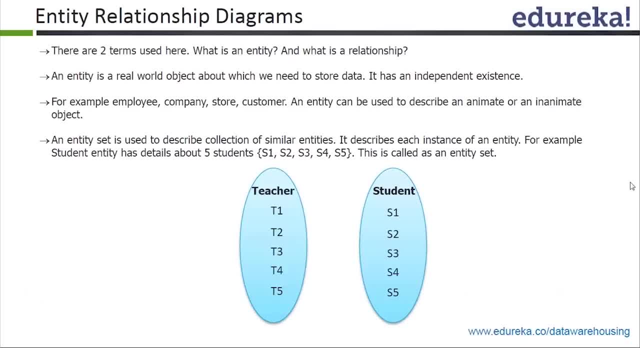 So what exactly this situation says is that if he would have built a mall, maybe he would have seen the proper exit strategy for his mall. So what exactly this situation says is that if he would have built a mall, maybe he would have seen the proper exit strategy for his mall. 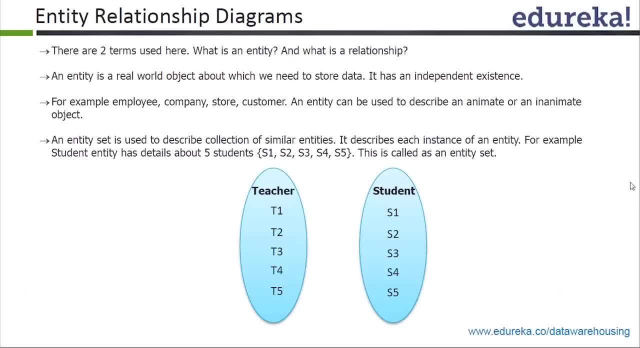 So what exactly this situation says is that if he would have built a mall, maybe he would have seen the proper exit strategy for his mall. So what exactly this situation says is that if he would have built a mall, maybe he would have seen the proper exit strategy for his mall. 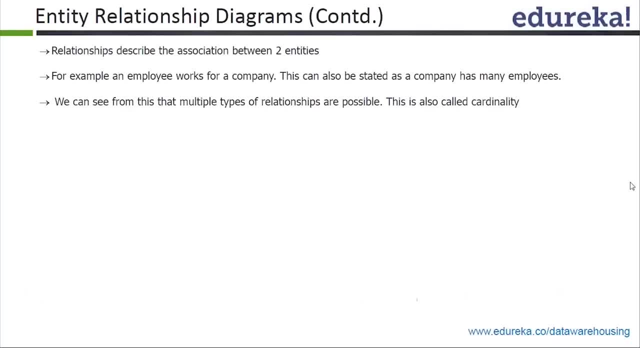 So what exactly this situation says is that if he would have built a mall, maybe he would have seen the proper exit strategy for his mall. So what exactly this situation says is that if he would have built a mall, maybe he would have seen the proper exit strategy for his mall. 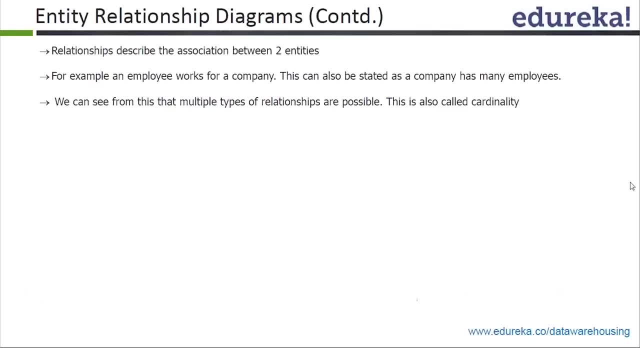 So what exactly this situation says is that if he would have built a mall, maybe he would have seen the proper exit strategy for his mall. So what exactly this situation says is that if he would have built a mall, maybe he would have seen the proper exit strategy for his mall. 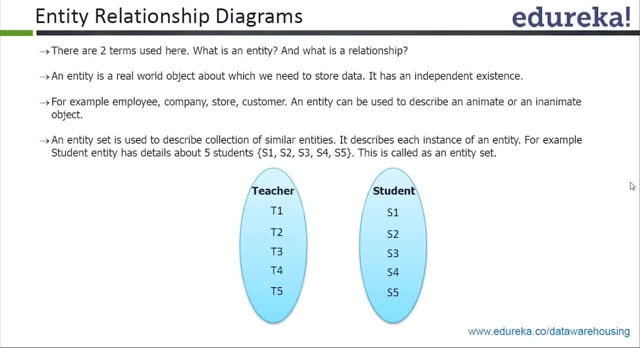 So what exactly this situation says is that if he would have built a mall, maybe he would have seen the proper exit strategy for his mall. So what exactly this situation says is that if he would have built a mall, maybe he would have seen the proper exit strategy for his mall. 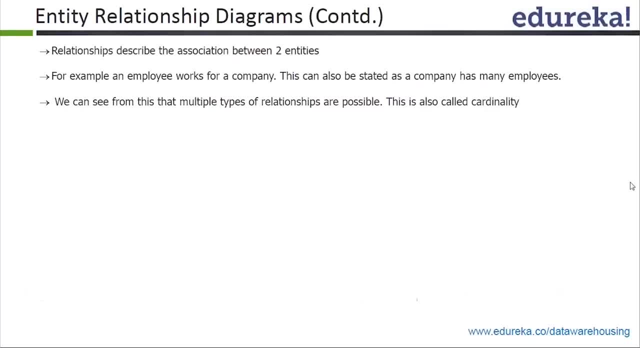 So what exactly this situation says is that if he would have built a mall, maybe he would have seen the proper exit strategy for his mall. So what exactly this situation says is that if he would have built a mall, maybe he would have seen the proper exit strategy for his mall. 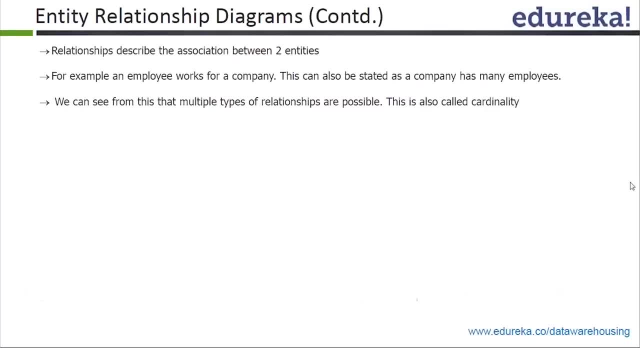 So what exactly this situation says is that if he would have built a mall, maybe he would have seen the proper exit strategy for his mall. So what exactly this situation says is that if he would have built a mall, maybe he would have seen the proper exit strategy for his mall. 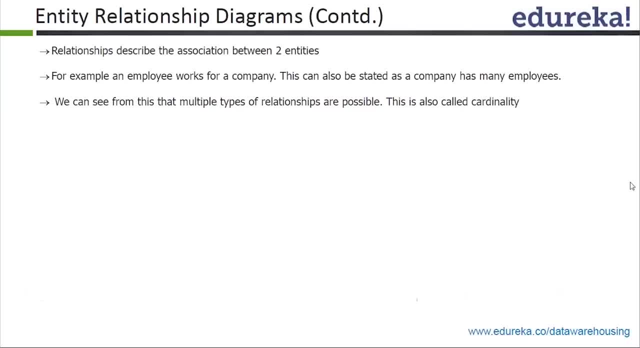 So what exactly this situation says is that if he would have built a mall, maybe he would have seen the proper exit strategy for his mall. So what exactly this situation says is that if he would have built a mall, maybe he would have seen the proper exit strategy for his mall. 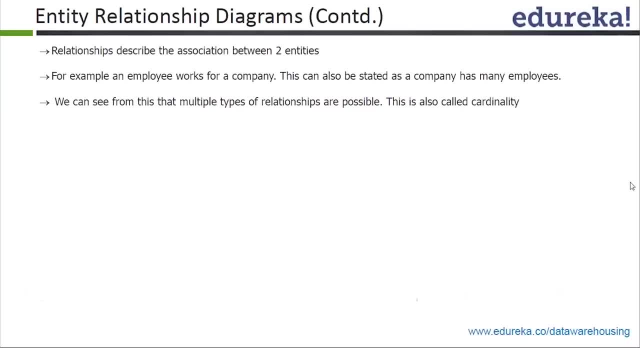 So what exactly this situation says is that if he would have built a mall, maybe he would have seen the proper exit strategy for his mall. So what exactly this situation says is that if he would have built a mall, maybe he would have seen the proper exit strategy for his mall. 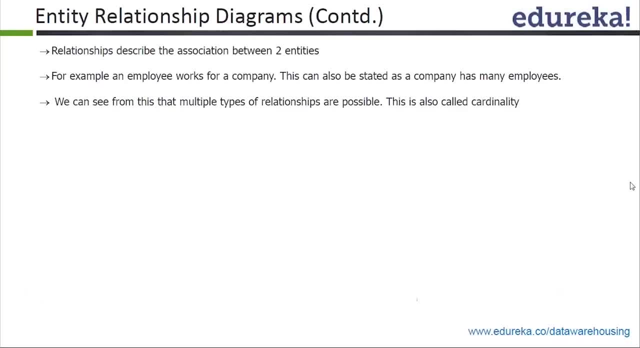 So what exactly this situation says is that if he would have built a mall, maybe he would have seen the proper exit strategy for his mall. So what exactly this situation says is that if he would have built a mall, maybe he would have seen the proper exit strategy for his mall. 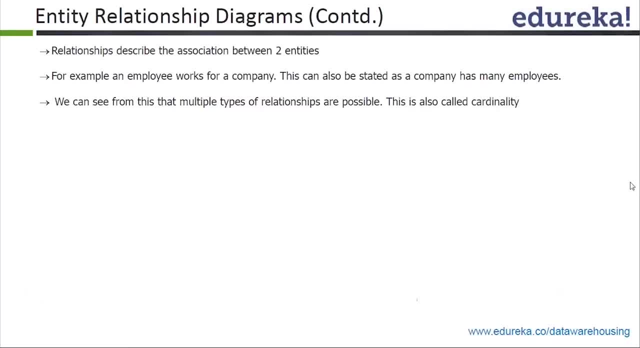 So what exactly this situation says is that if he would have built a mall, maybe he would have seen the proper exit strategy for his mall. So what exactly this situation says is that if he would have built a mall, maybe he would have seen the proper exit strategy for his mall. 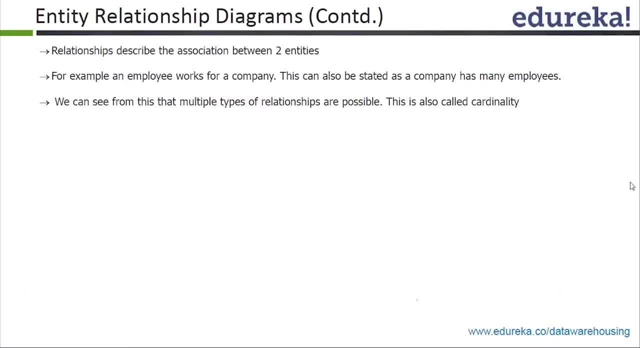 So what exactly this situation says is that if he would have built a mall, maybe he would have seen the proper exit strategy for his mall. So what exactly this situation says is that if he would have built a mall, maybe he would have seen the proper exit strategy for his mall. 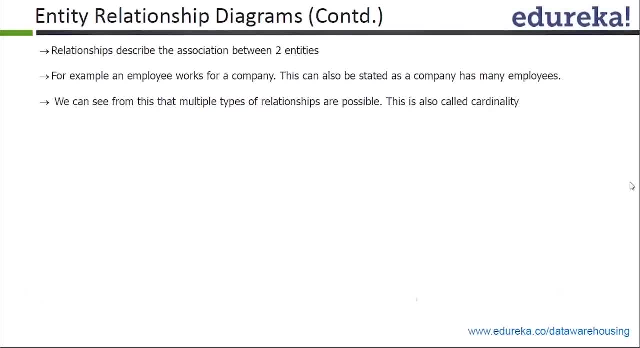 So what exactly this situation says is that if he would have built a mall, maybe he would have seen the proper exit strategy for his mall. So what exactly this situation says is that if he would have built a mall, maybe he would have seen the proper exit strategy for his mall. 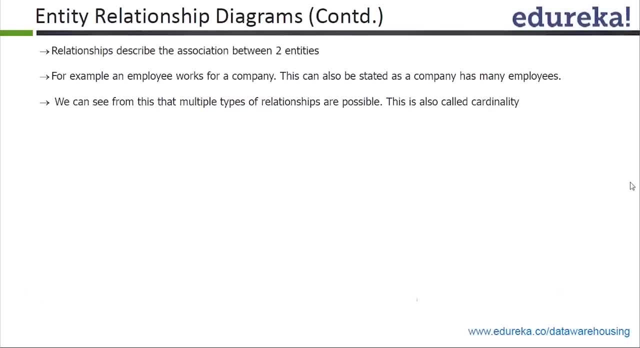 So what exactly this situation says is that if he would have built a mall, maybe he would have seen the proper exit strategy for his mall. So what exactly this situation says is that if he would have built a mall, maybe he would have seen the proper exit strategy for his mall. 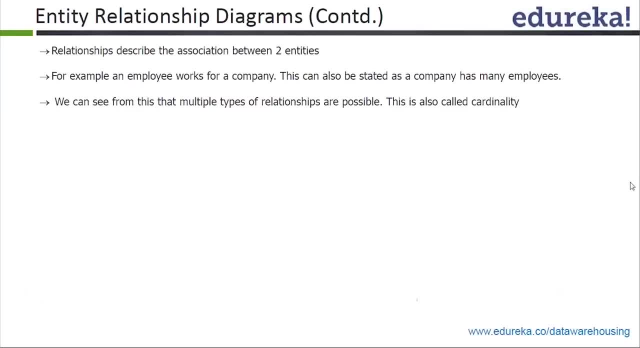 So what exactly this situation says is that if he would have built a mall, maybe he would have seen the proper exit strategy for his mall. So what exactly this situation says is that if he would have built a mall, maybe he would have seen the proper exit strategy for his mall. 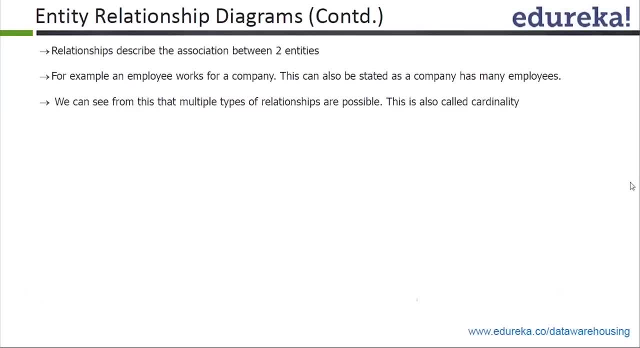 So what exactly this situation says is that if he would have built a mall, maybe he would have seen the proper exit strategy for his mall. So what exactly this situation says is that if he would have built a mall, maybe he would have seen the proper exit strategy for his mall. 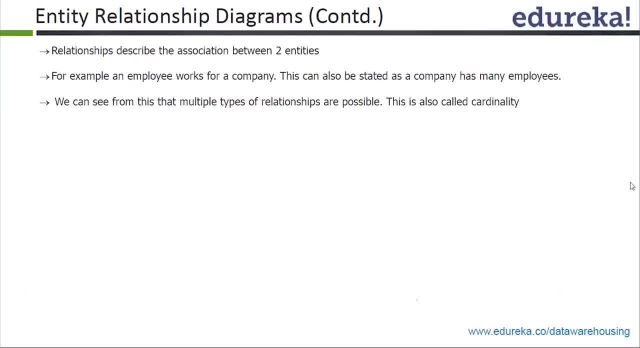 So what exactly this situation says is that if he would have built a mall, maybe he would have seen the proper exit strategy for his mall. So what exactly this situation says is that if he would have built a mall, maybe he would have seen the proper exit strategy for his mall. 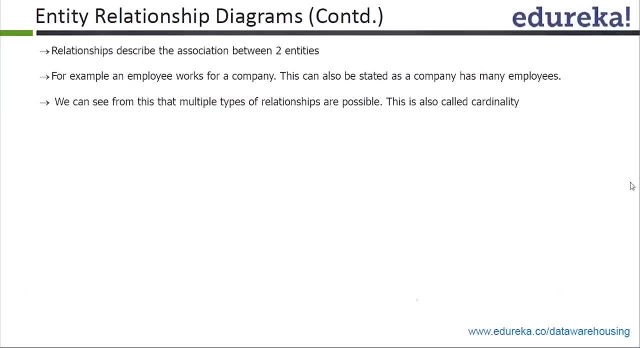 So what exactly this situation says is that if he would have built a mall, maybe he would have seen the proper exit strategy for his mall. So what exactly this situation says is that if he would have built a mall, maybe he would have seen the proper exit strategy for his mall. 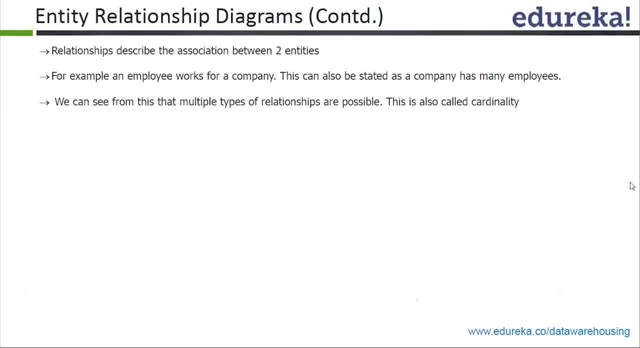 So what exactly this situation says is that if he would have built a mall, maybe he would have seen the proper exit strategy for his mall. So what exactly this situation says is that if he would have built a mall, maybe he would have seen the proper exit strategy for his mall. 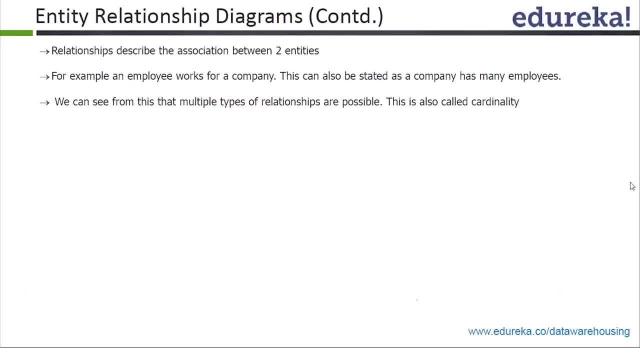 So what exactly this situation says is that if he would have built a mall, maybe he would have seen the proper exit strategy for his mall. So what exactly this situation says is that if he would have built a mall, maybe he would have seen the proper exit strategy for his mall. 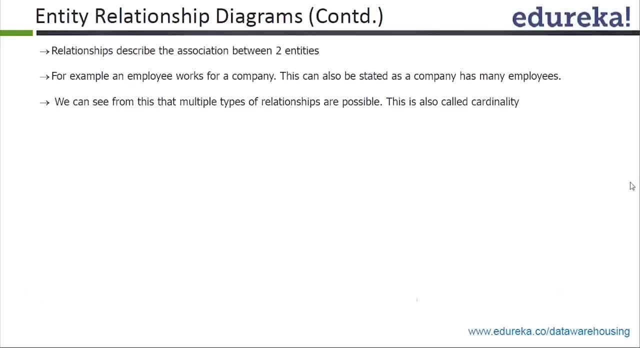 So what exactly this situation says is that if he would have built a mall, maybe he would have seen the proper exit strategy for his mall. So what exactly this situation says is that if he would have built a mall, maybe he would have seen the proper exit strategy for his mall. 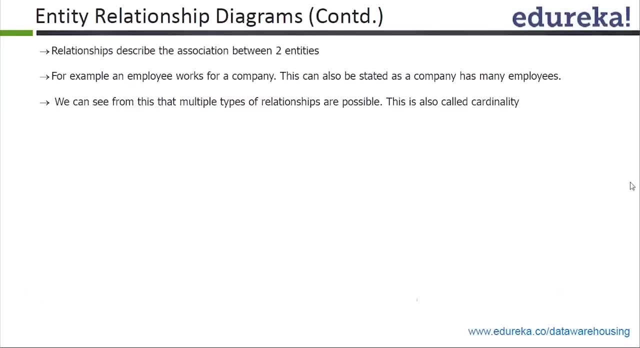 So what exactly this situation says is that if he would have built a mall, maybe he would have seen the proper exit strategy for his mall. So what exactly this situation says is that if he would have built a mall, maybe he would have seen the proper exit strategy for his mall. 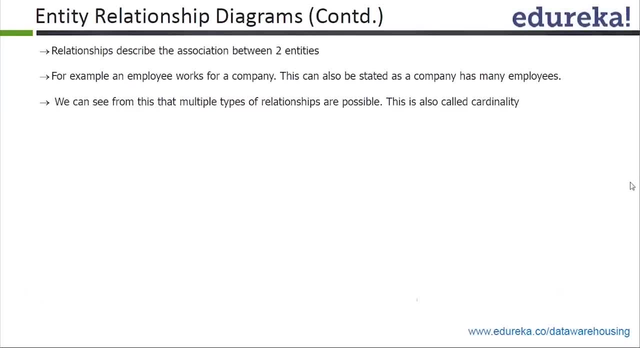 So what exactly this situation says is that if he would have built a mall, maybe he would have seen the proper exit strategy for his mall. So what exactly this situation says is that if he would have built a mall, maybe he would have seen the proper exit strategy for his mall. 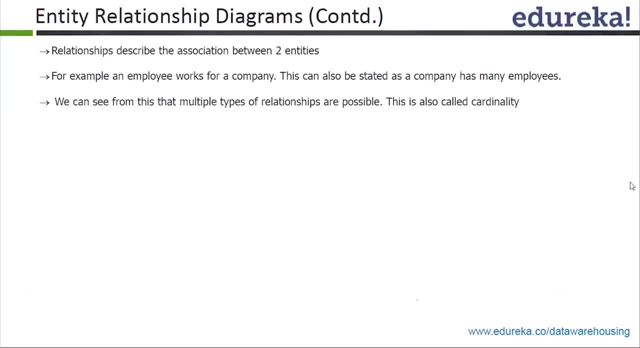 So what exactly this situation says is that if he would have built a mall, maybe he would have seen the proper exit strategy for his mall. So what exactly this situation says is that if he would have built a mall, maybe he would have seen the proper exit strategy for his mall. 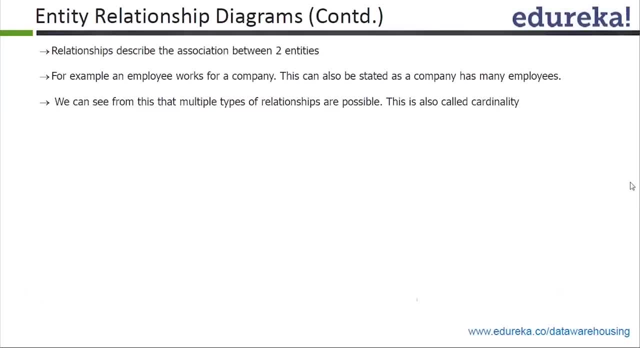 So what exactly this situation says is that if he would have built a mall, maybe he would have seen the proper exit strategy for his mall. So what exactly this situation says is that if he would have built a mall, maybe he would have seen the proper exit strategy for his mall. 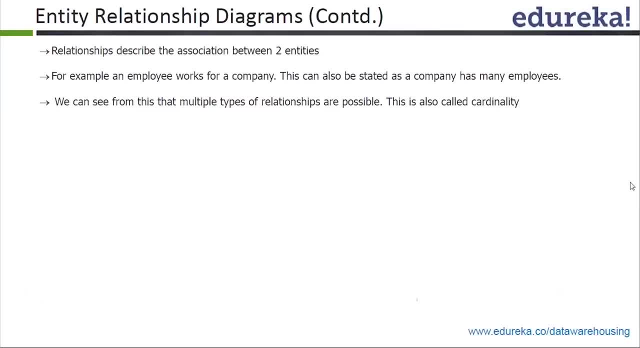 So what exactly this situation says is that if he would have built a mall, maybe he would have seen the proper exit strategy for his mall. So what exactly this situation says is that if he would have built a mall, maybe he would have seen the proper exit strategy for his mall. 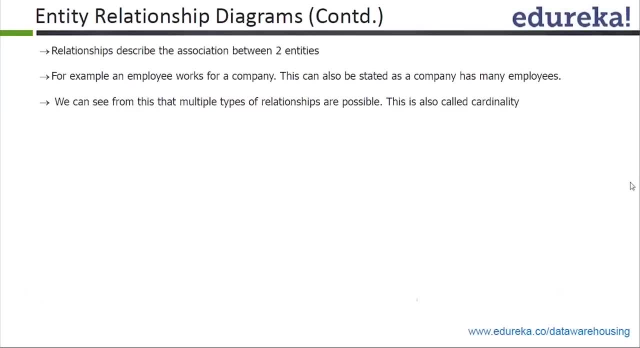 So what exactly this situation says is that if he would have built a mall, maybe he would have seen the proper exit strategy for his mall. So what exactly this situation says is that if he would have built a mall, maybe he would have seen the proper exit strategy for his mall. 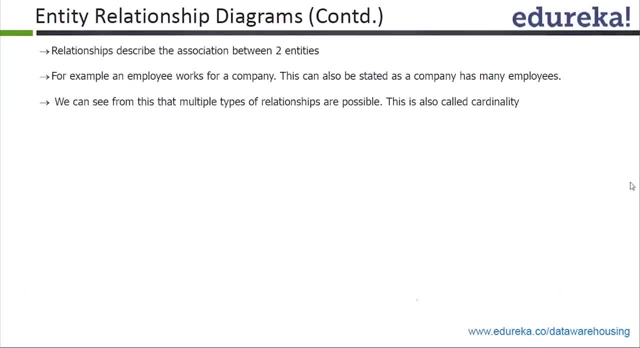 So what exactly this situation says is that if he would have built a mall, maybe he would have seen the proper exit strategy for his mall. So what exactly this situation says is that if he would have built a mall, maybe he would have seen the proper exit strategy for his mall. 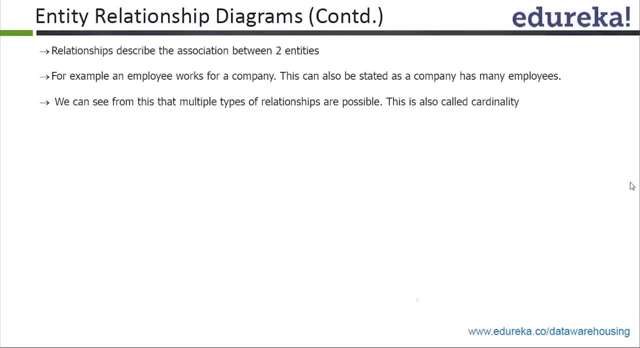 So what exactly this situation says is that if he would have built a mall, maybe he would have seen the proper exit strategy for his mall. So what exactly this situation says is that if he would have built a mall, maybe he would have seen the proper exit strategy for his mall. 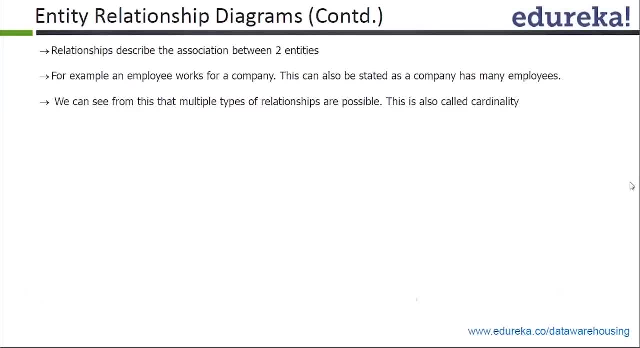 real world like, like, for example, the teacher right, a teacher can have many students. for example, in a school there is only one teacher, but there are many students. so a teacher can have many students, but a student can have only one teacher. so so the relationship between teacher to student is one to many. so 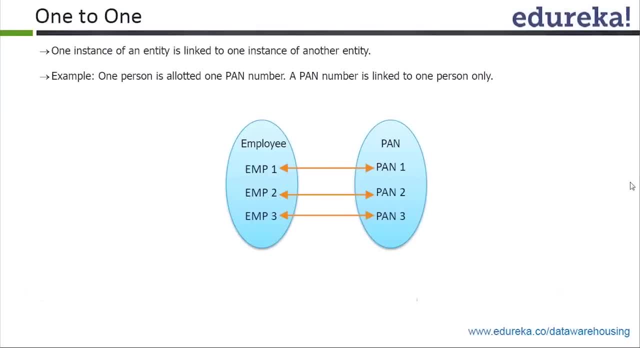 that's what I mean, that this type of relationship is called cardinality. so yeah, so the first type of relationship is one-to-one relationship, in which a each, each element in one entity is related to only one element in the other entity, and vice versa. so, in this case, an employee. 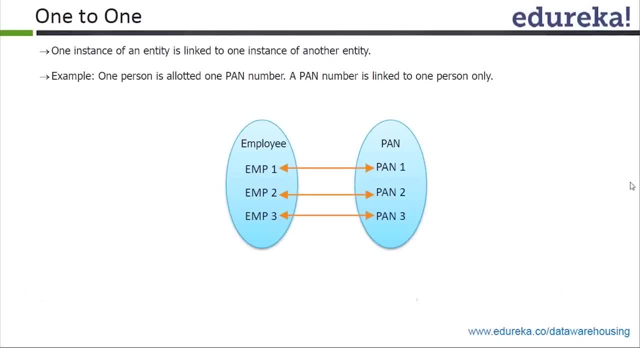 there is an employee entity and there is a pan entity. pan entity is just entity which is a person, so between including and fruit- and in this case is a person- is um, as a janitor. so yeah, so there are a few different relationships there. and as a 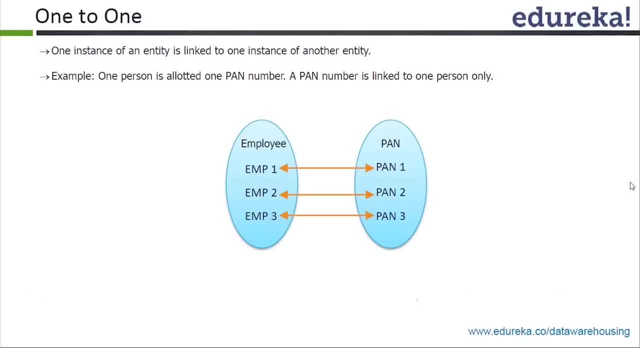 single or a two Coke example, any, every kind of business in the same place. here is it stores the PAN card number or whatever. but let's take an example, relevant example, like there's an employee entity and say there is another entity which is, say, a department entity, so one employee can only belong to one. 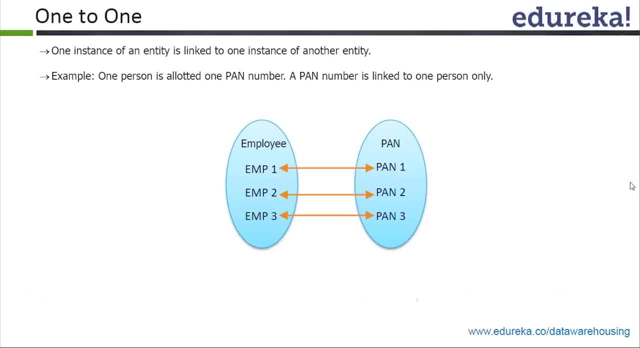 department and one. sorry, this is not correct for the one-to-one. so let's say passport number, so similar to PAN number, right one? one employee can have only one PAN number and one PAN number can only be related to one Empire. so in this case a both the entities have one-to-one relationship between them self and sorry. 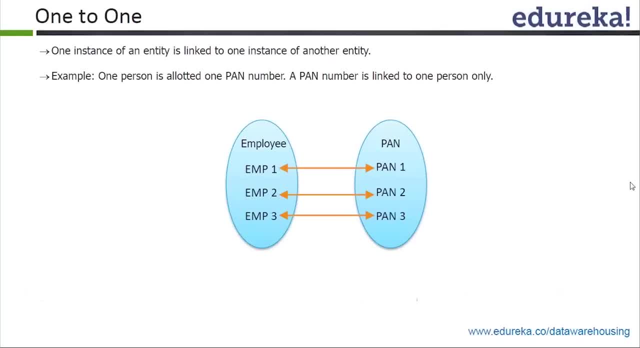 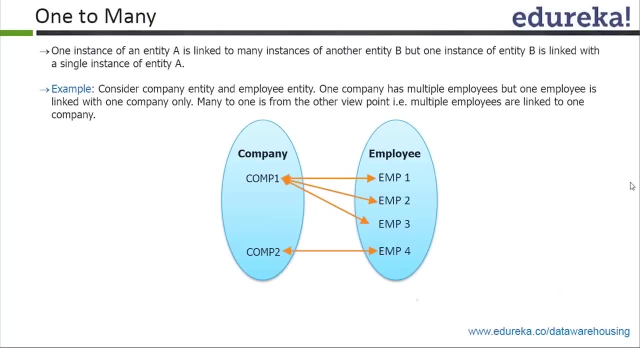 and instance in an entity has one-to-one relationship with the instance in another entity, so that is one-to-one. the next type of cardinality is one to many. in this case, as the name suggests you, one entity from sorry. one instance from one entity is related to many instances in the other. 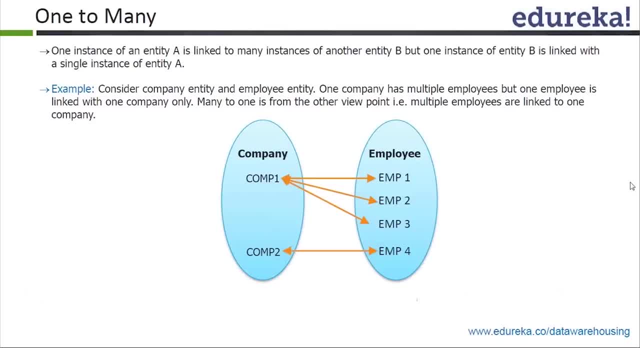 entity. so in this case, the example which is shown here, there is one company which has company one which has three employees: employee one, two and three. so one company from the company entity has many employees but one employee from the employees entity has only one company related to it. So this type of relationship where 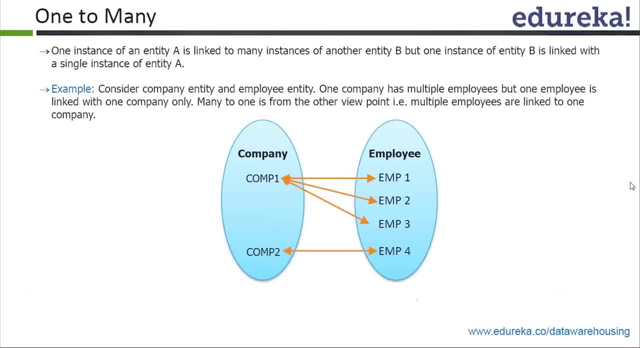 one instance of an entity A is linked to many instances of another entity B, but one instance of entity B is linked with a single instance of entity A is called one to many relationship. so in this case there is a one too many relationship from company to employee. 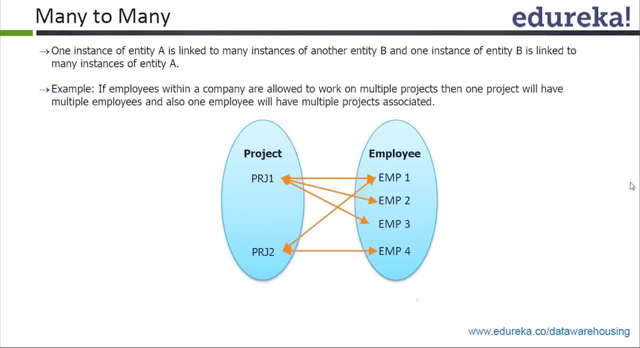 so that is one-to-many relationship. the next one is many to many. so in this case, as you see in the example, there is a project entity and there is a employee entity, so one employee can work for different projects. so in this case employee one is working for both- project one and project two- but employee and 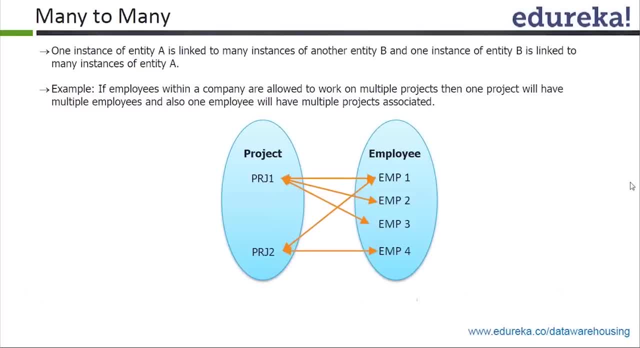 one project can have multiple employees, obviously. so in this case there is a many to many relationship between the two entities. so a many to many relationship is a relationship in which one instance of an entity A is linked to many instances of another entity B and one instance. 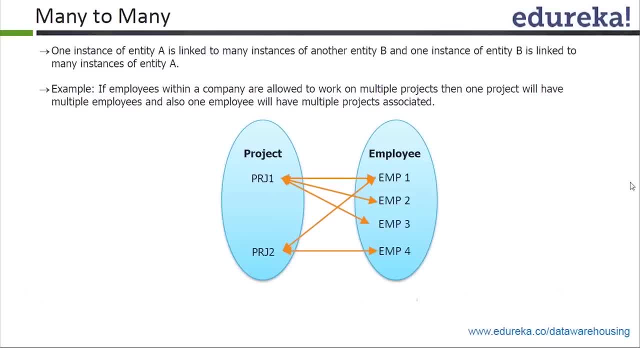 of entity B is linked to many instances of entity A, so it's both sides. they are related, many to many, so that is many to many relationship. so these are three different types of cardinalities. one to one, one too many, oh many so many. so that's about the relationship between the 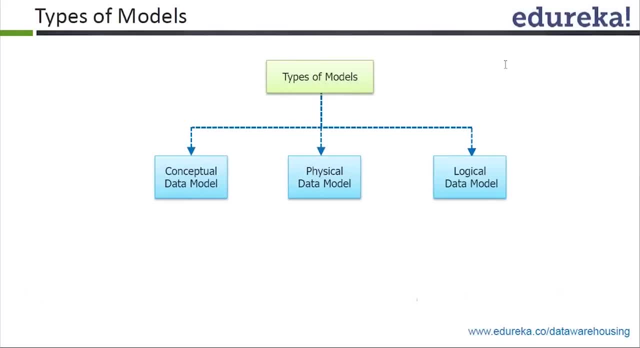 entities. the next topic we are going to discuss is the different type of models which you can represent. using your different type of models you can have before you build the data system warehouse so, as I told you before they, they can be the first step to build a. 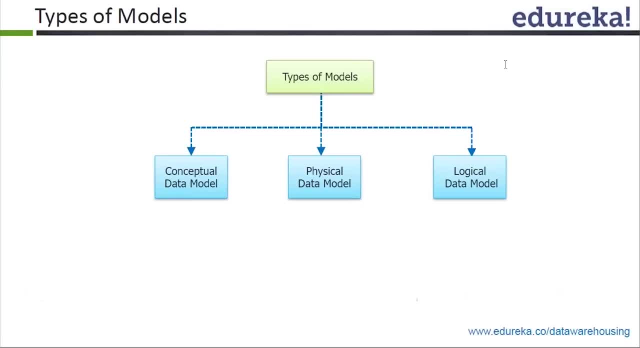 data warehouse is a conceptual data model, then you have a logical data model, then finally you have a physical data model. so this is the different types of data models. you can have it's different types of blueprint which is meant for different audiences. so we will see in the slides coming. forthcoming slides. 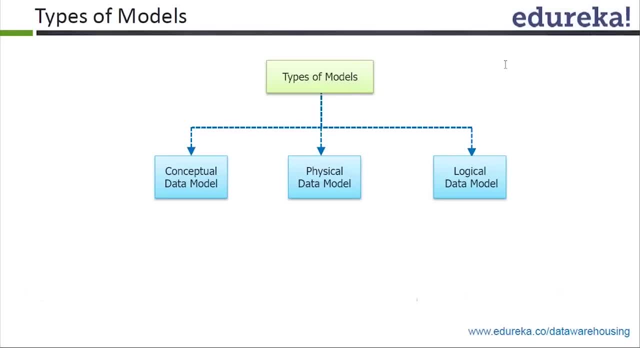 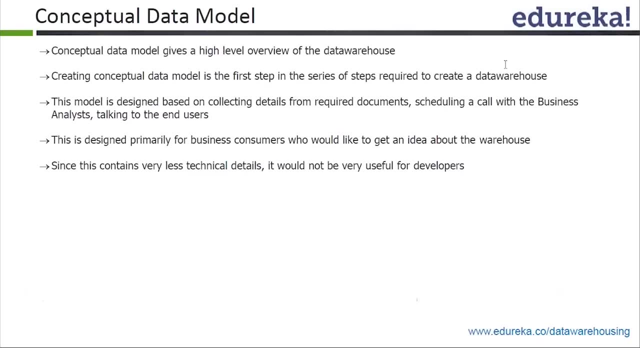 what are these models and why are these built and who is the target audience for all these data models? so, as I said, the first model which we built for a data warehouse is a conceptual data model. as the name suggests, it's just a concept of your data warehouse, so it gives you a very high level overview of your data. 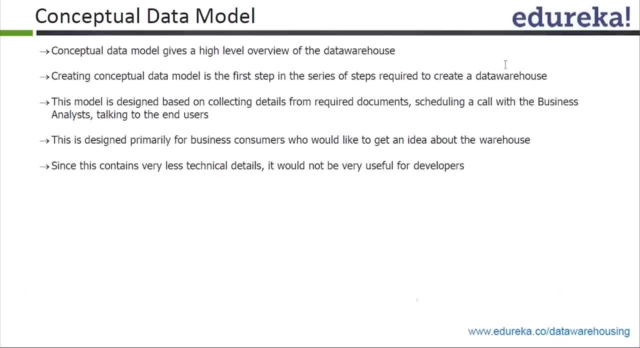 model, creating a conceptual data model, is the first step. as I said, it's the first step in creating your data warehouse. this model is designed based on collecting requirements from the client, from the, from the users. then you discuss with your, your counterparts, your client counterparts, and you discuss with your. 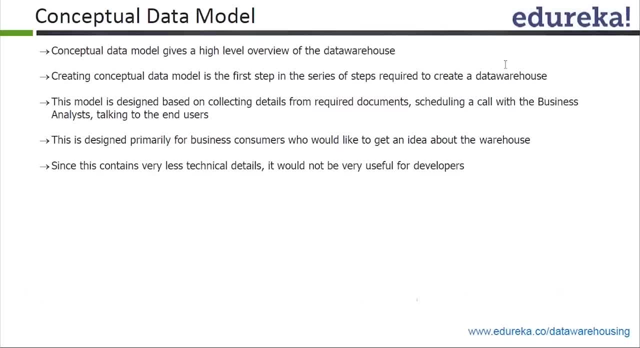 business users and about the requirements and the reports, requirements which they have. based on, that you actually build is conceptual data model. so once you develop this conceptual data model, which will be in a very simplistic manner so that even users and consumers, the consumers and the business users from your side can understand, so once this is 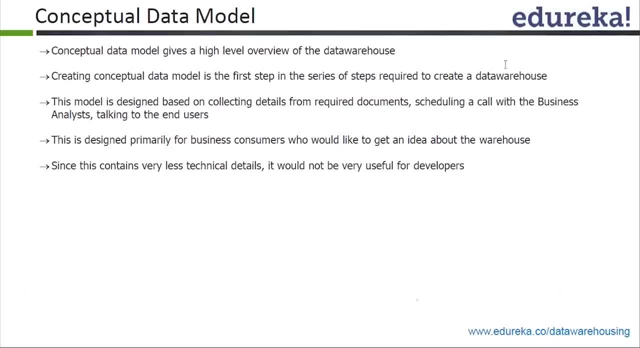 developed, then you will share the details with. you will share the details with the users and once it is confirmed and both of the client and the modeler is confirmed that have the same understanding, then you will proceed with the other data models. If it is not approved, then you will stick with the conceptual data model and then correct. 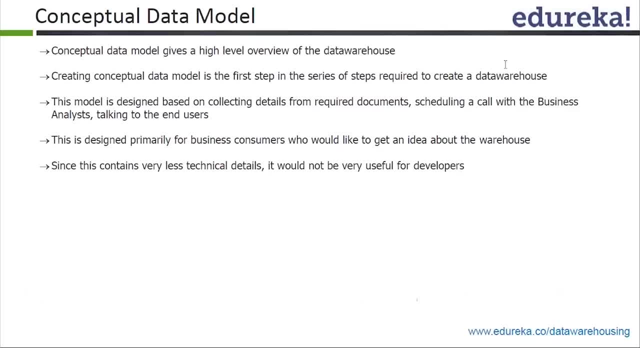 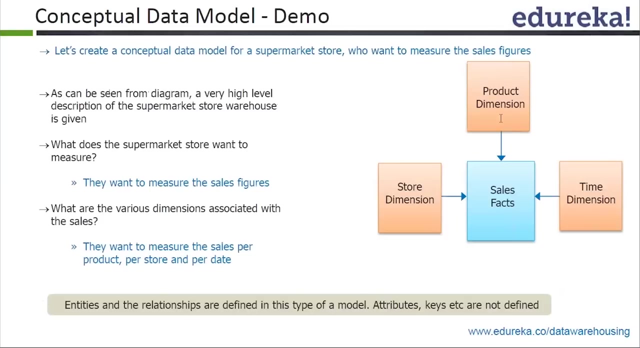 your conceptual data model before you move on to build your logical data model. So this is the first step. This will not have any technical details inside. It will not be very useful for your developers. It will just give you a business overview. So this is a sample conceptual data model which you see here in this slide. 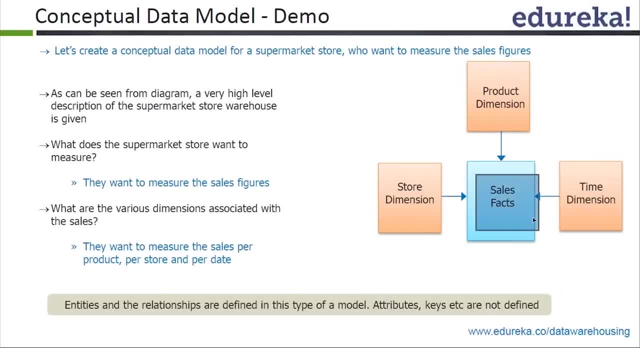 There is a simple sales fact table and then there are three dimensions: product dimension, store dimension, time dimension. So once you So looking at this conceptual data model, you can say that you have a sales fact table and the sales fact entity, you have a product dimension entity, you have a store dimension. 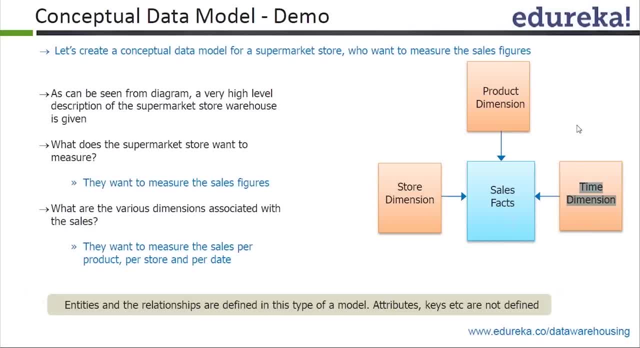 You have these three dimensions and one fact table, and each dimension is related to this fact table. That is it. That is simple information you can get from this conceptual data model. So this is very high. It doesn't show. It doesn't show you what different measures your fact table has or how these tables are. 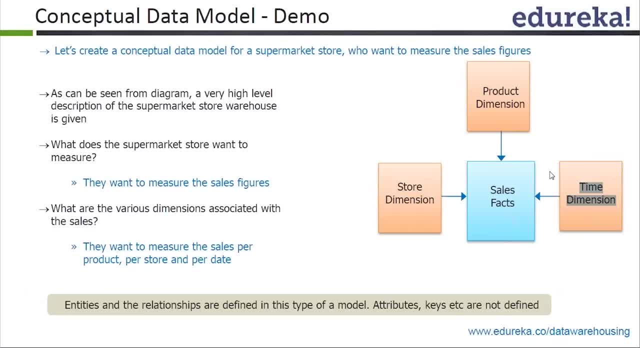 related Nothing. So it just gives you there are four tables and they are related to each other. So this particular conceptual data model is for a supermarket. which who wants to measure the sales fact? I think this example we discussed a lot of times. 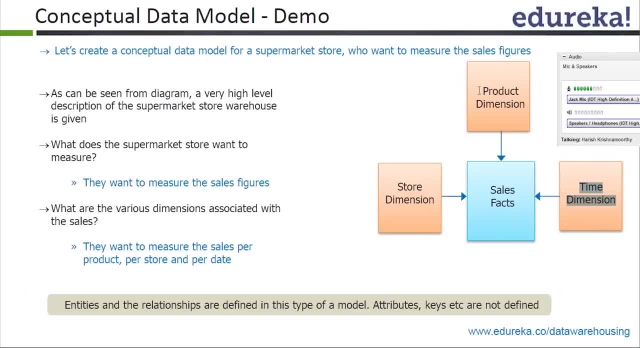 So These are. this conceptual data model was come up by asking questions. the client like: what exactly you want to measure? The client said: we want to measure the sales figures, So we put a sales fact and then they ask the question: what are the various dimensions associated? 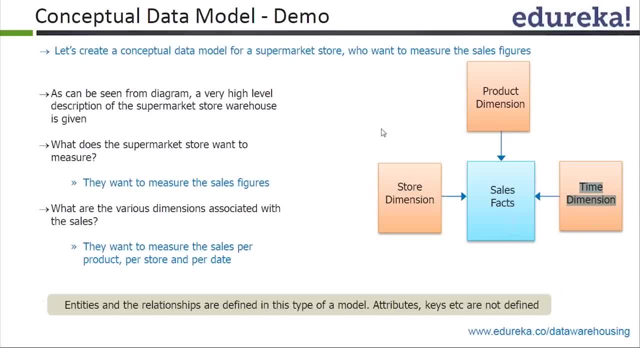 with this sales fact. So this conceptual model which I am, which is shown in this slide, is come up by asking questions like what to the clients, Like what does the supermarket store want to measure? So by that we came up with the sales fact. 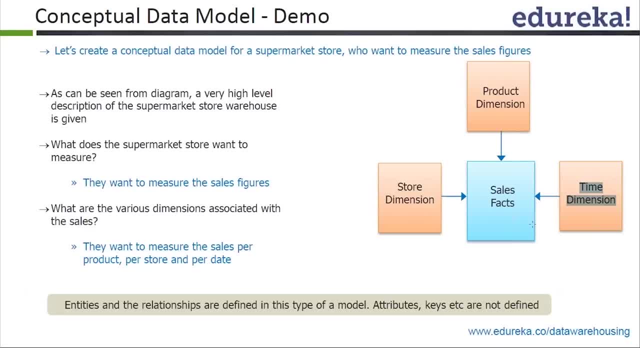 The client said they want to measure sales figures. So we had a sales fact. inside this conceptual model, What are the various dimensions associated with the sales fact? What different dimensions in which you want to see the sales fact bifurcated? in what different? 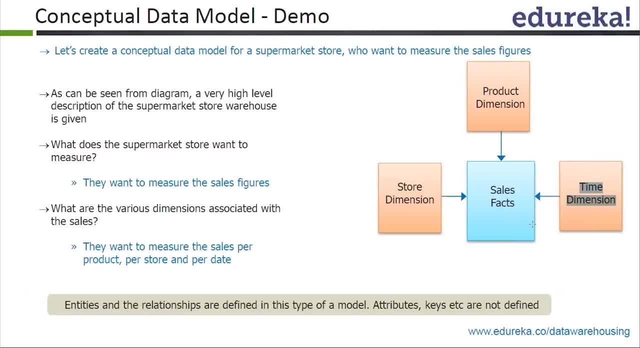 dimensions. So they wanted to measure the sales by customer, by product. So you added different dimensions. So this particular diagram, This entity, The entity and the relationship are defined in this year in this diagram, but the attributes, keys etc. As I said, is not defined. 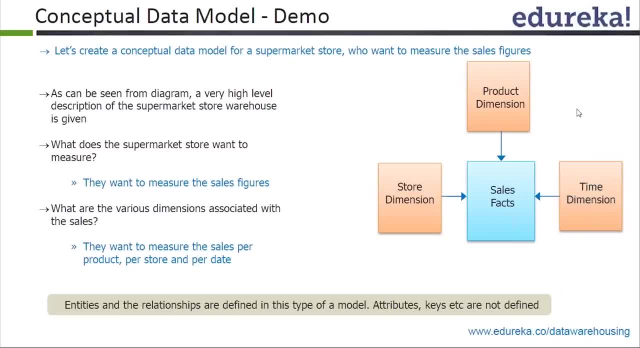 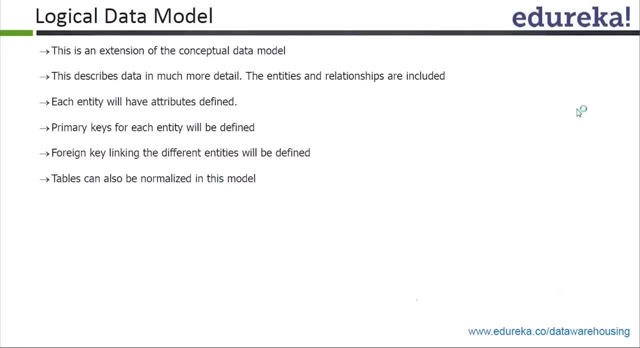 So this will just give you a basic overview of the data model. The next data model which we will deep dive into, after the conceptual data model, is logical data model. So the logical data model. It actually contains more information and more technical information than your, not really. 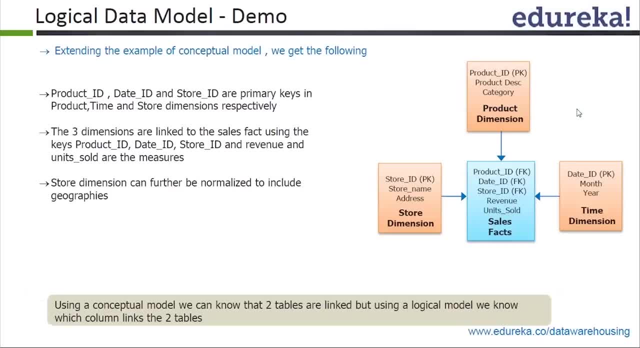 I won't say technical, but it has more information than your conceptual data model. This is an extension of a conceptual data model. This describes more about your entities, different entities you have in your data model. This will tell you, define the. this will define the relationship. 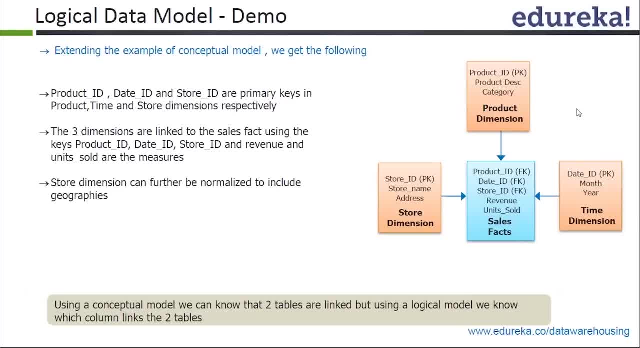 What kind of? what columns are involved? attributes are involved within the entities. What attributes actually relate these two entities? What is the primary key? foreign key, linkages, What are the? and also different. you can see different dimensions in your model being normalized into other dimensions. 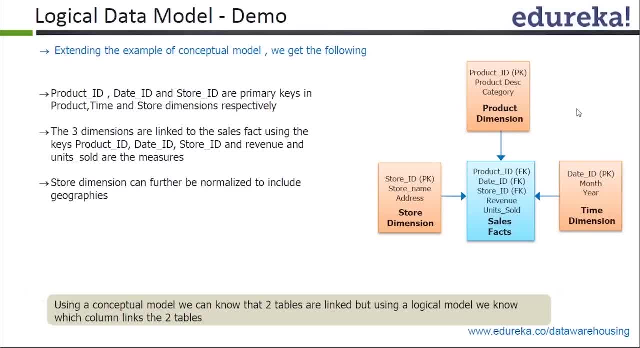 But in your conceptual model You will only see A concept of your dimension. you won't see that. OK, this dimension, How the dimension information is stored in the logical model. Is it normalized? the data is it? is the data being split into different tables, or what? 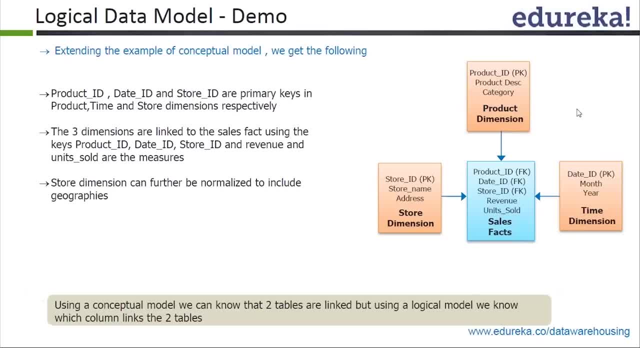 you won't actually see that in your conceptual model. you will only see that in your logical model, where they will say: OK, we have two different tables, which is shown, which is actually storing the dimension, this dimension data. So this level of information you will see in the data model, but still, I would say it. 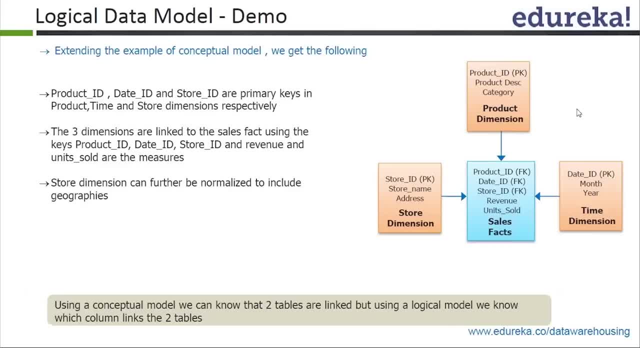 will not have Information for the developers to start developing. So this conceptual model will definitely give you different attributes. like you see, in this diagram There is a. you will show you what different primary keys it has, what different relations. what is the column which is responsible for the relationship between the two? 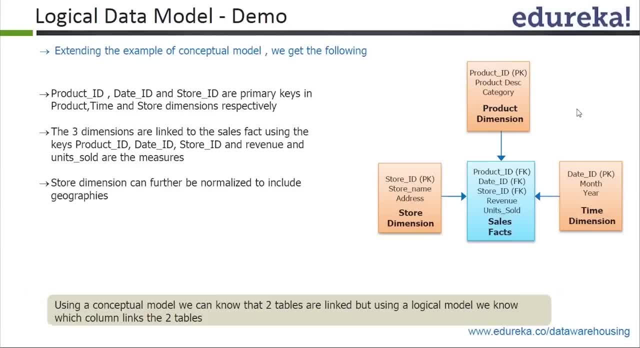 So this is the conceptual model. So this is the conceptual model. So this is the conceptual model. So between the two tables and you will see the relationship between shown, You will see the measures and the Different columns in a particular table, but still you can't, you don't have. 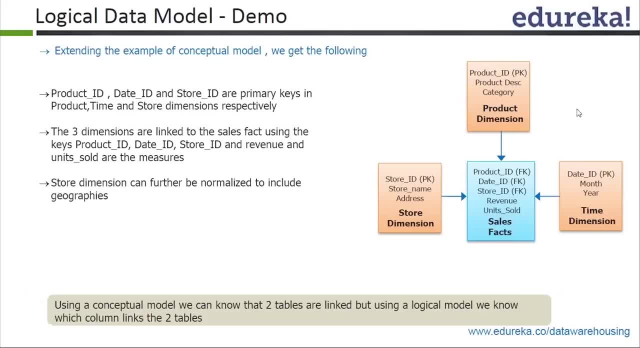 The exact information for the developers to develop. so this representation is still not for the developers, but it's just a logical data model. It will show you different tables, different columns involved in the table and then the relationship between these tables. So The example you see here. 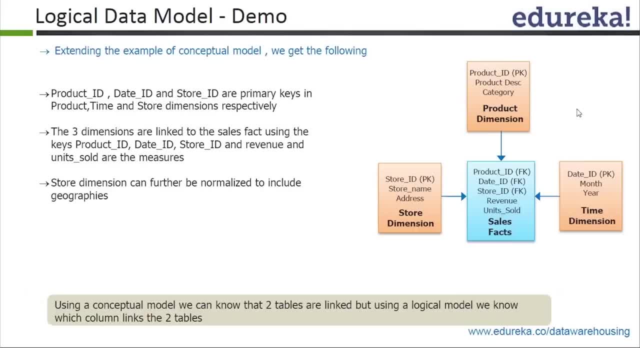 there is a product dimension, store sales fact and time dimension. so they you see what is the primary key for each dimension and for the, and different foreign keys in your fact table and different attributes in your fact table. so this is what is a logical model, but it's still not informative enough for 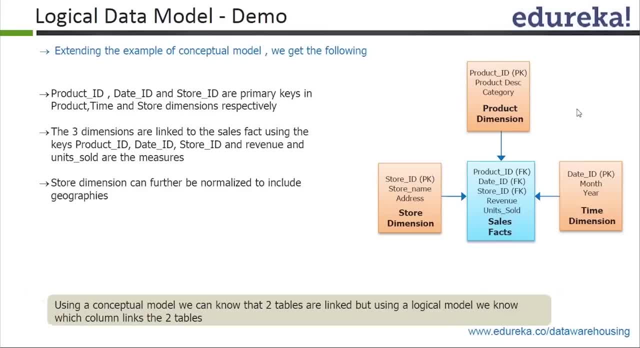 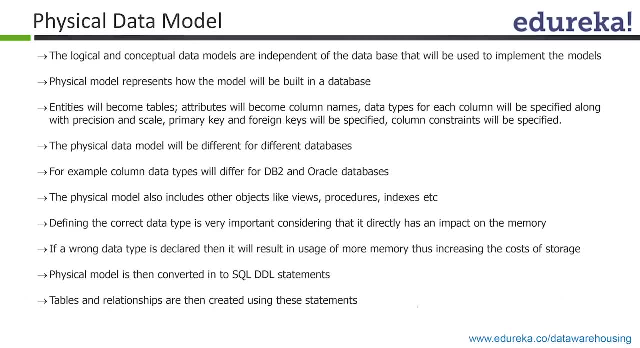 the developers to start implementing. so the next one is the physical data model, which is actually the representation of your physical database, which you have formed or designed. this is one step further with the logical model. so in the logical model, you saw that you, you already know what are the columns. you 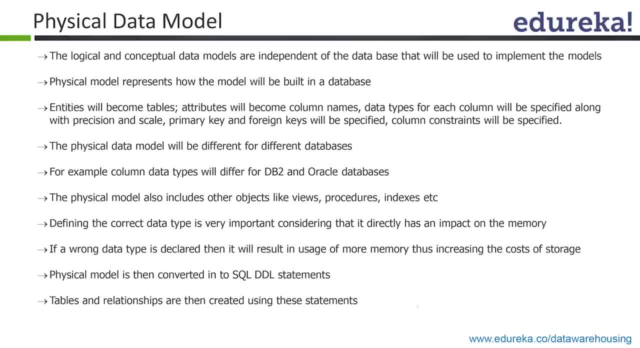 already know what are the attributes related. so not the columns but the attributes related. you already know the different tables in your data data model, but in physical data model you will actually see what are the data types of these different attributes. what is the primary key constraint, what are the different constraints on your particular? 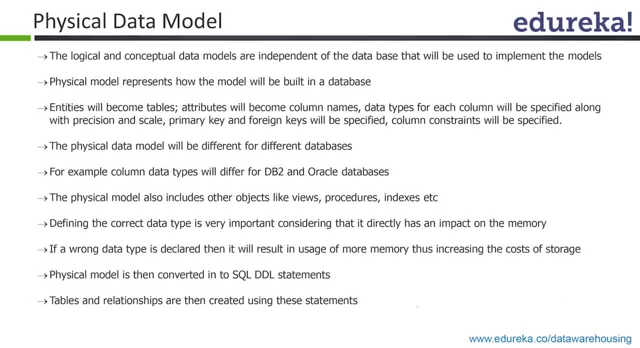 table. everything related to your table and the data model will be put in this table, put in this shown in this model where, by looking at this data model, you can actually write SQL scripts, BDLs, to create the physical tables in your database. so it will have all the information. 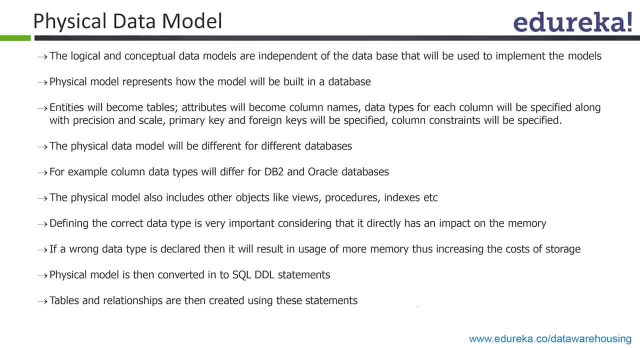 so, for example, if entities will become from conceptual data model to logical data model, the entities will still the term we use in the conceptual and and the logical data model for is entities and attributes. but as soon as you move from logical data model to physical data model, the term entities become stables. 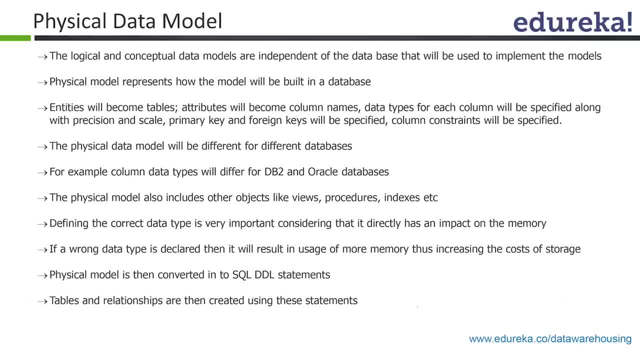 attributes will become columns and you will have data types associated with each column. you will have all the physical primary keys, foreign keys defined, column constraints defined. so, and also because you are defining everything which is for a database, it will always depend on the underlying database you are using, like, for example, the data types in Oracle and db2. 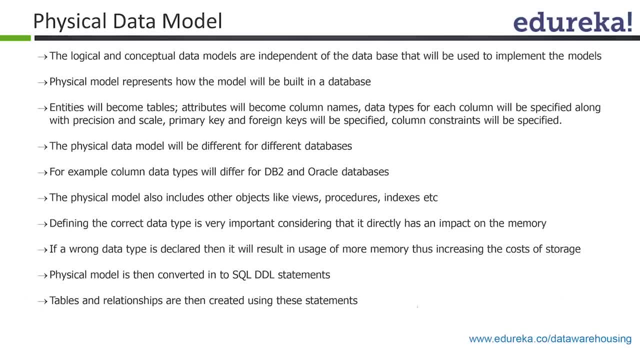 might be different. so in Oracle may be used. we use worker in db2. you might use some other terminology for the same character data type so you can have different representation for different databases. so physical data model will actually be different for different database. but logical- excuse me- logical data model and conceptual data model doesn't depend on. 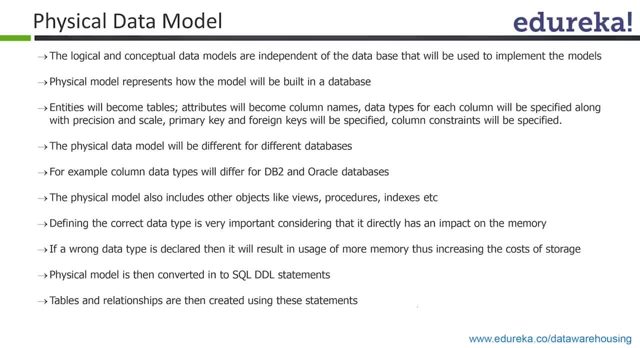 the underlying database. so you will. so you will define a physical data model in such a way that a developer can look at your physical data model, can and actually write sequence statement onto your database and create the physical objects. so this is the data model which is necessary and this is the data model. 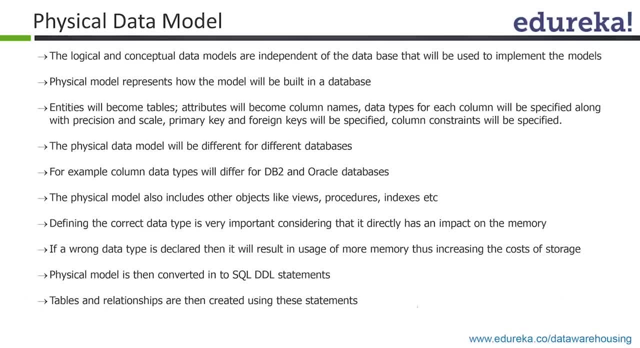 which is necessary for a developer to proceed and create is physical tables and relationship, physical relationship indexes, everything. everything will be in this physical data model, table space and all the technical details. so that is the final data model we'll arrive at after performing or folder, after going step by step from conceptual to logical and from logical to physical. 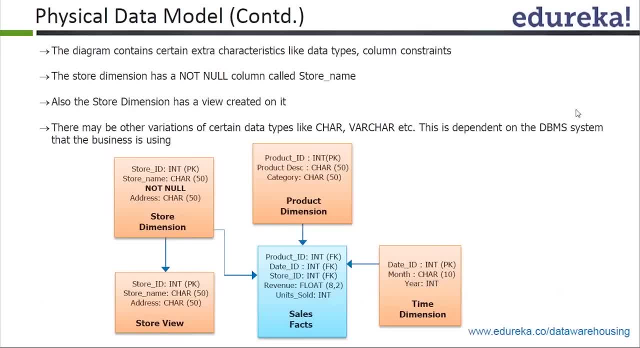 So this is a sample how your physical data model will look like. So you can see, in this physical data model you can actually see the constraints on dimension table- stored dimension table, where you see there is a constraint- not null constraint- on a particular column, which is store name. 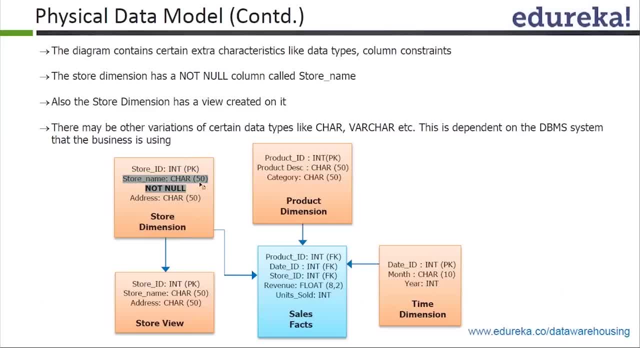 So, which means that store name cannot be null. So, and you can see the data type defined for each column, which is char 50 for store name, char 50 for address, and then you can also see the primary key defined on these tables, Similarly, for all other tables, the data types defined, the constraints defined, the relationship. 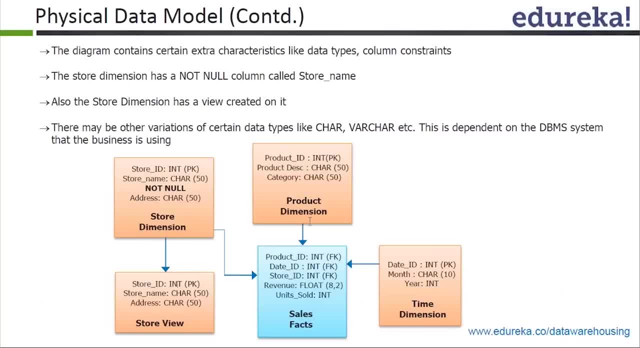 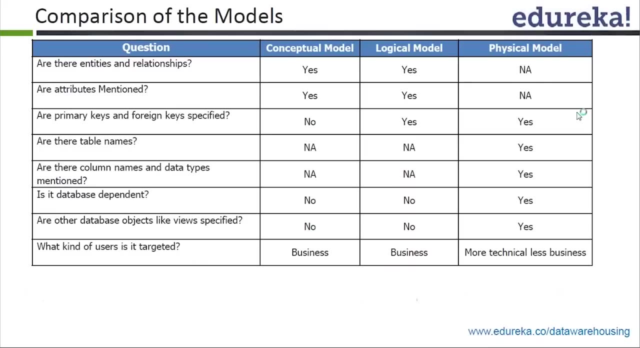 defined. So your physical data model will show everything related to your data, Your tables. so this is where your entities become tables and attributes becomes columns. So that's about the three different data models, but let's look at this before we move further. let's look at the comparison tables, just to give us more understanding of these different 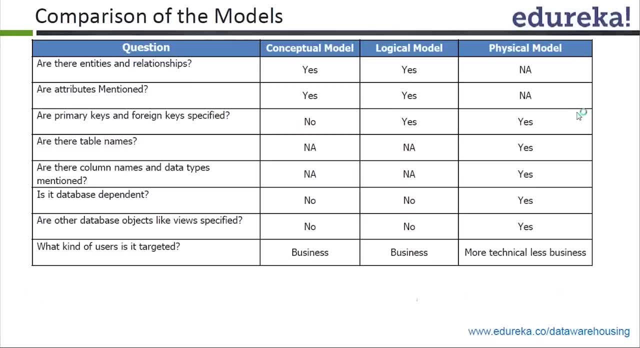 models. So let's see, let's look at the left side question And imagine we have these questions on the left side. So let's see what is the answer to these questions in yes or no in these different data models? So are the entities and relationship shown in conceptual data model? 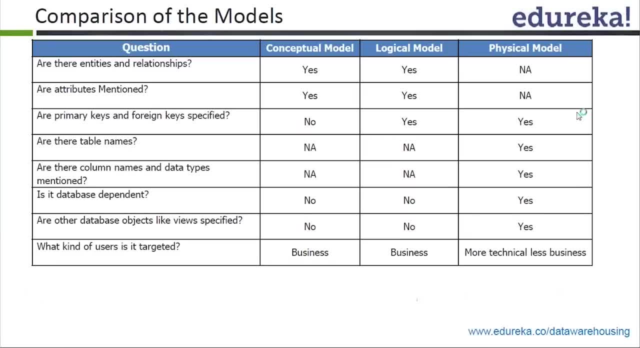 Yes, you can see the entities and relationships In a logical data model. yes, you can see the entities and relationship in a logical data model. In a physical data model it's not applicable. Why it is not applicable? Because in a physical data model there is no entities and relationship anymore. 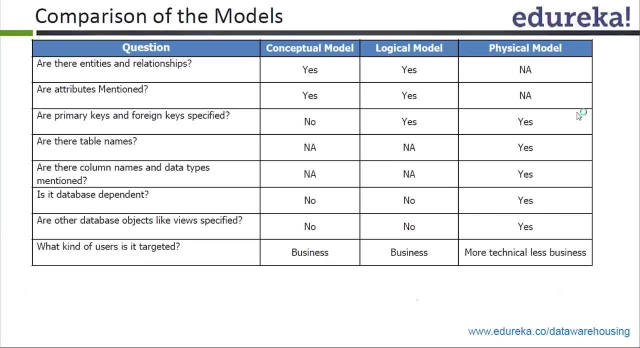 It is tables and the integrity constraints and database constraints, So the terminology changes from logical to physical. So there is this particular concept of entity and relationship is not applicable in the physical data model. Similarly, attributes: Are the attributes mentioned? Yes, Conceptual. 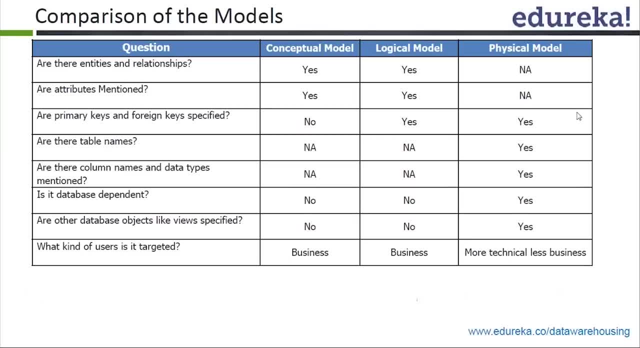 Yes, Logical, Yes, But in a physical data model this is not applicable, like this previous case. What about the primary keys and foreign keys? So the conceptual data model doesn't give you this information about primary keys, as we discussed. So it will only give you the entities and then it will give you the relationship. 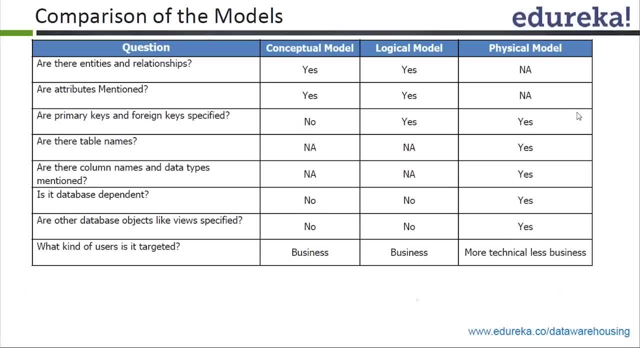 It won't give you the columns which are responsible for foreign keys. Okay, But your logical data model, yes, it will give you, And your physical data model, yes, it will give you foreign key relationship. What is the column or the attribute responsible for that relationship? 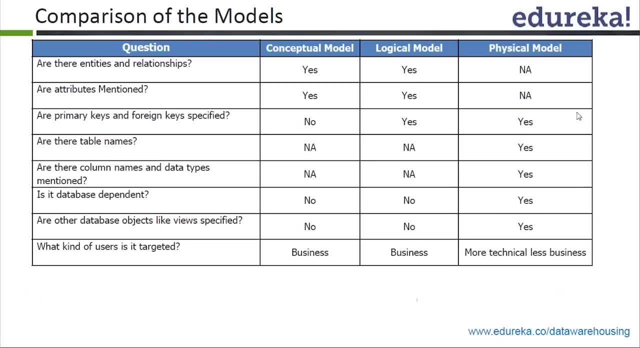 So are there table names in the conceptual data model? No, Because there are no tables. There are only entities and relationship in a conceptual model. Logical data model: No, It is not applicable actually for both conceptual and logical, because until then there is no. 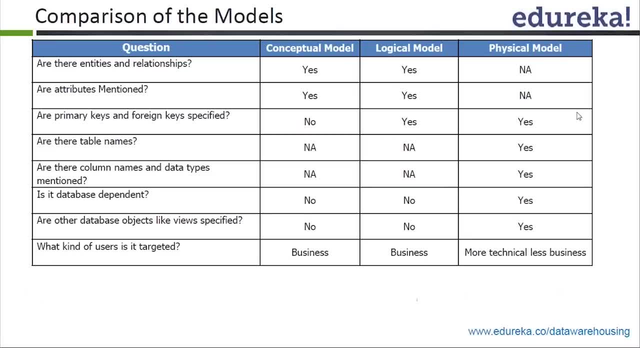 bifurcation of entities and relationship as tables and columns, And are the column names and data types mentioned? No, They are not mentioned in the first two, logical and conceptual. It is only mentioned in the physical data model. Is this database? is it a database dependent? 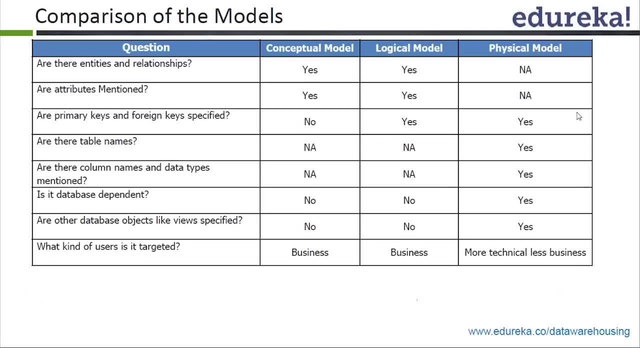 Is it database dependent? Okay, As I discussed, conceptual and logical data model does not depend on the underlying database. We are going to build the actual database. But physical data model depends on the underlying database because different database softwares can have different data types and so on and so forth. 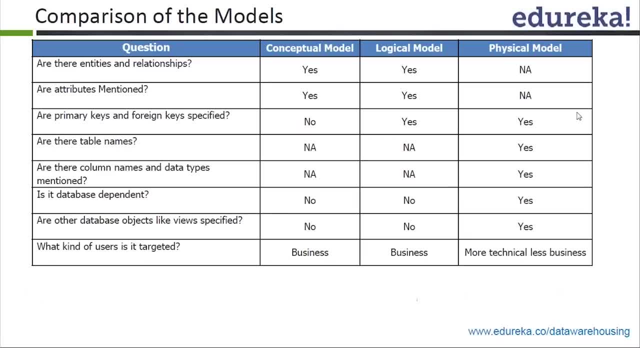 Are other database objects, like views, specified in the conceptual data model? No, As I said, there will be only entities. in the conceptual data model There are no tables, no views, no database objects In logical data model, also no database objects.